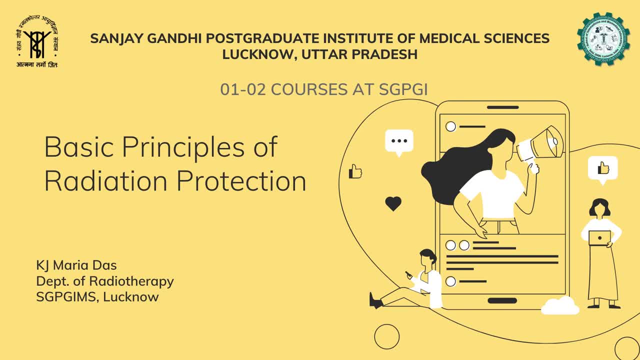 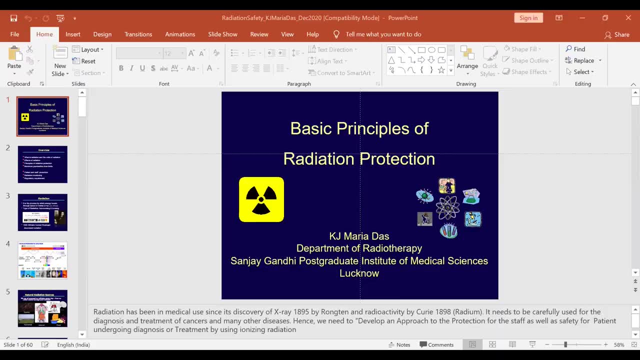 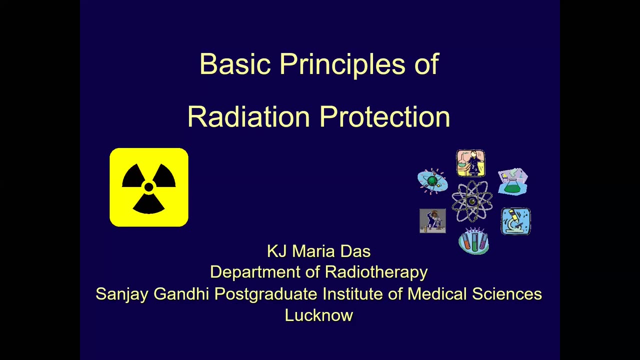 Good evening to everyone. So today I will be talking about the radiation principles and radiation protection. We all know 1985 X-ray was discovered by Ronjan, which was an accidental discovery, But it had a great application because those days when they had to cut open, 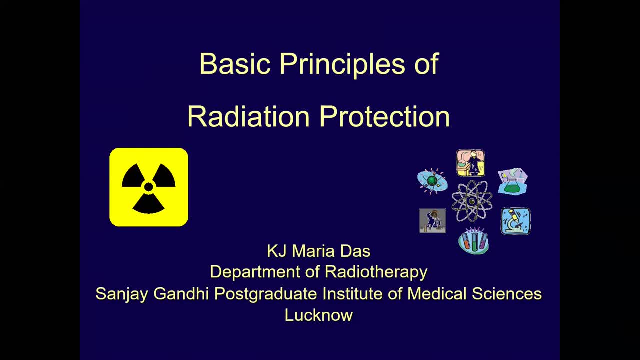 something to see what is happening inside. they were able to visualize the bone lung, for example, pneumonia or etc. So it was a great discovery in that way to know, and they named the name as X-ray, basically because they could see what was not visible to human. 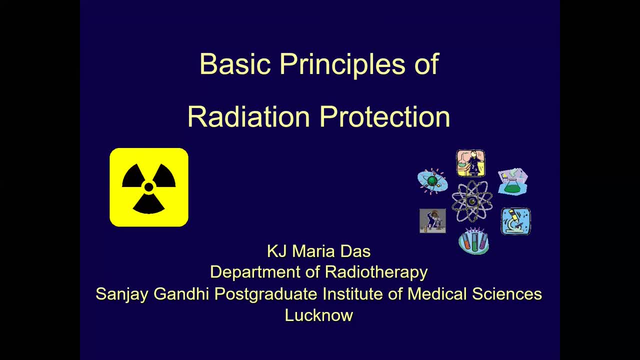 eye inside the body, which is bone and soft tissues, they could visualize it. So X-ray is dangerous, is hazardous, but is it really? Up to what extent and what kind of a risk is it? For example, safety and precautions makes the justification that the benefit is large compared. 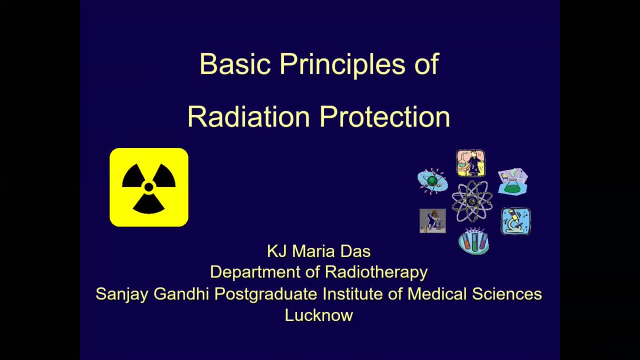 to the small damage. So that way of judicial justification- benefit versus risk ratio- helps us to justify and keep using it. However, it is mandated that we have to understand the basic principles so that we always caution about it and we know exactly what to do. what 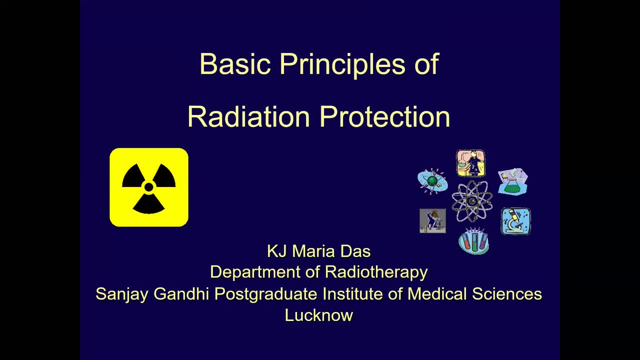 not to do. So that is what we are doing. So we are doing a lot of work to do that. What we are doing now is we are going to be doing something called the X-ray- X-ray to do So my lecture. I would like to cover you telling a very, very rough idea about what is. 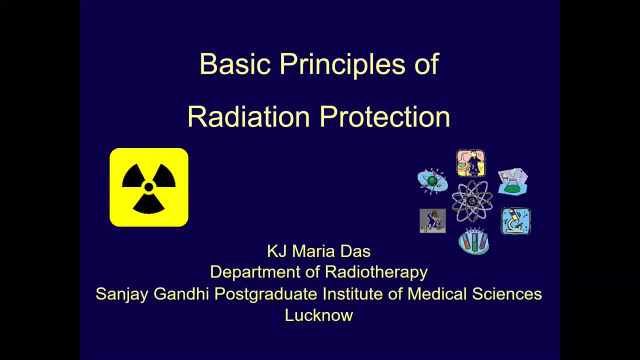 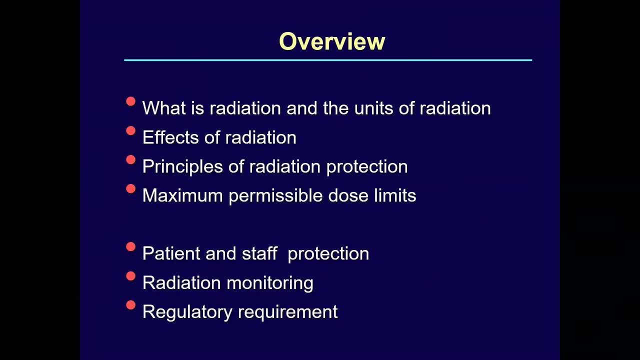 background radiation and how do we relate background radiation with medical radiations and what are the dose limits? what are the dose limits and what are the radiation units generally we use? because if we don't know the unit then we cannot respect whether we are talking in. 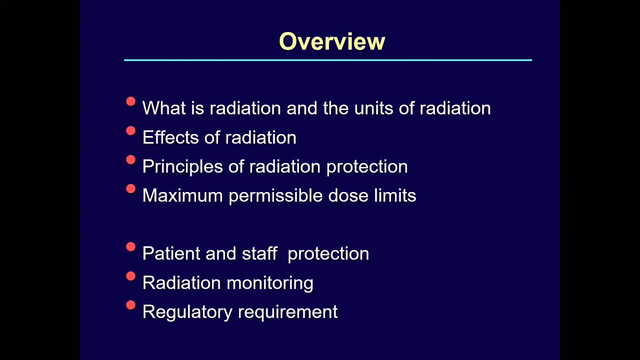 millimeter or centimeter- we should know what does the millimeter or centimeter means- and international radiation councils and national councils, like the atomic energy regulatory board. they are stipulated guidelines and standards which we have to respect and practice and it is not an option, it's a mandatory. So I'm going to start my lecture talking about what is radiation, basically. 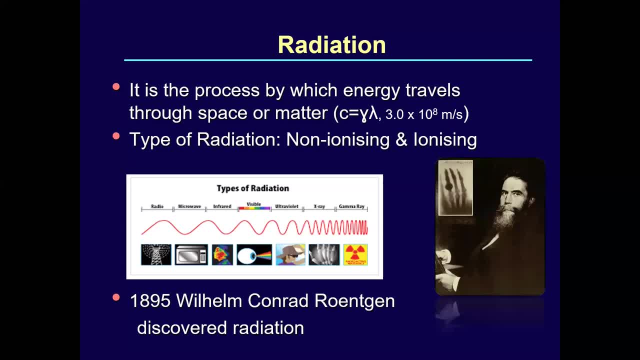 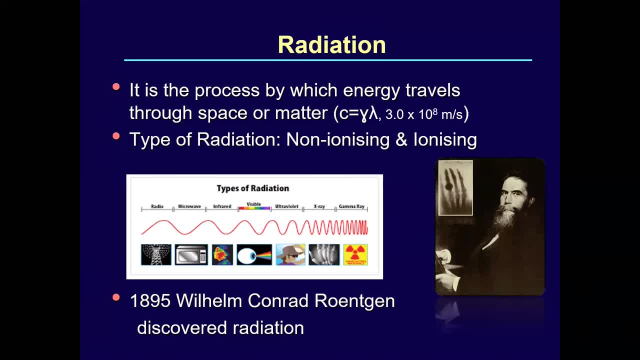 light, which is 3 into 10 to the power, 10 meter per second, And they have the same property which we call as electromagnetic properties, that they can be deflected by electric and magnetic fields and they have a transverse waveform And these wave radiations could. 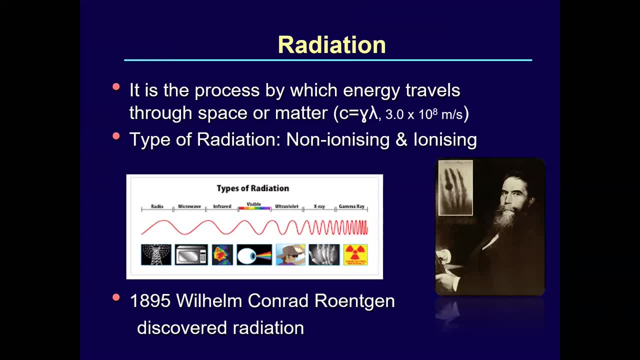 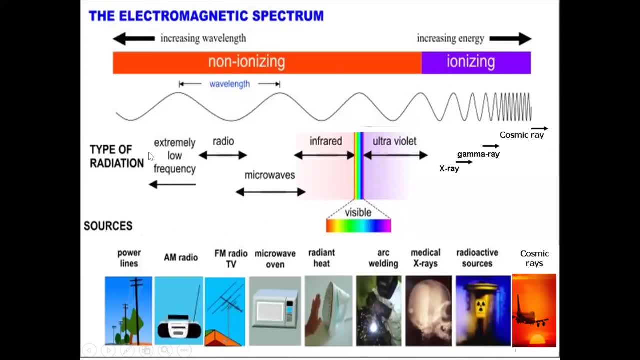 be ionizing and non-ionizing. So when you look into the spectrum of radiation, the non-ionizing part starts from the extremely low frequency radiations. What we mean is the frequency is less, then the wavelength is very large And it is non-ionizing. Radio waves, microwaves. 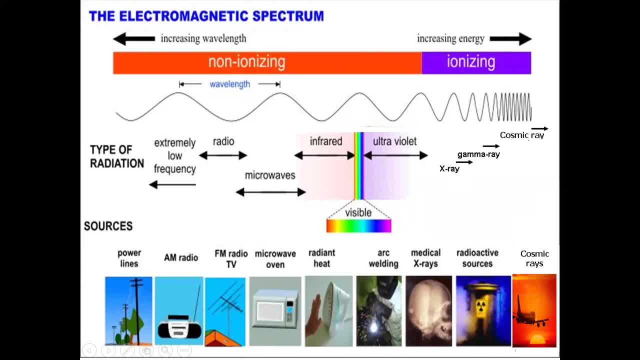 infrared and all these radiations are used in power lines: radio, what we are listening to, FM radios, microwaves, radiation, irradiators and all So up to this is fine, and then we have the visible light and ultraviolet radiation. Up to ultraviolet radiation, we have the visible. 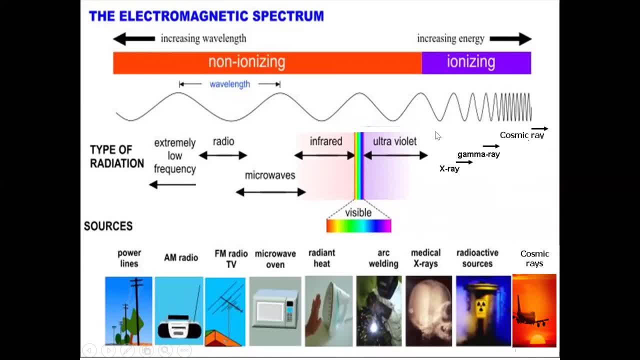 radiation. It is considered as non-ionizing radiation And beyond that, if you look into the thing, the frequency is indirectly proportional to wavelength and you could see that the wavelength, as ionizing radiation has an increasing energy. the wavelength keeps decreasing and as wavelength 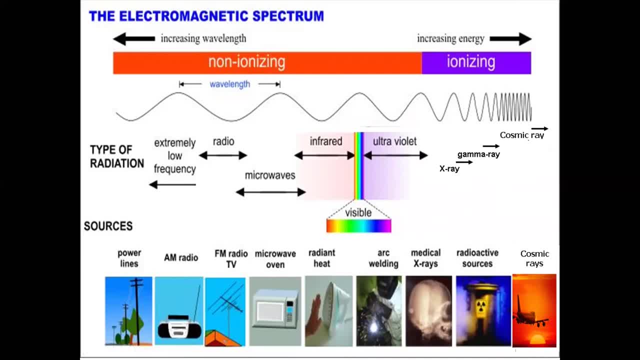 decreases, the frequency increases Because, you remember, C is equal to mu lambda and if you see, mu is equal to C by lambda. So the frequency and wavelength is always inversely proportional to each other. Now, with the ionizing radiation we have various 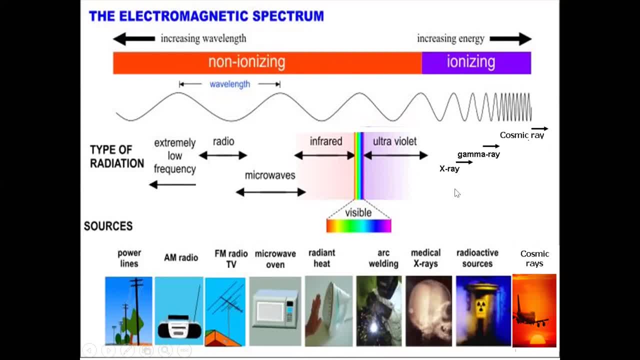 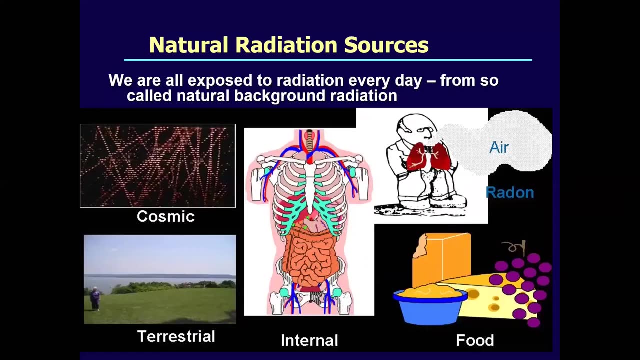 radiations like the X-ray, which is produced by man-made, and there are radioactive isotopes which are natural as well as man-made, and there are terrestrial cosmic radiations, which is always there in the cosmos, which we cannot get away from. So look into the natural radiation. 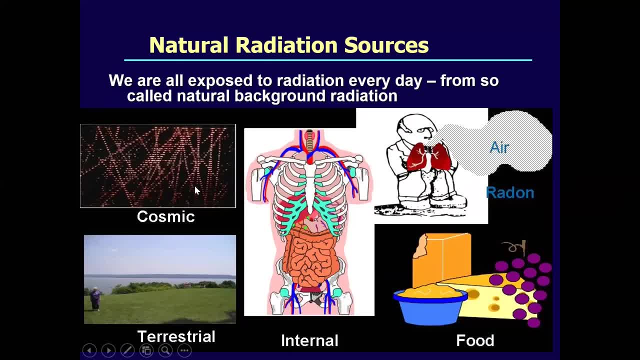 Natural radiation. the major radiation, natural radiation is from the cosmic radiation, which is from the terrestrial radiation. So the radiation is always there in the cosmic radiation Terrestrial, which is also non-uniform when they reach the earth. And there are lot of. 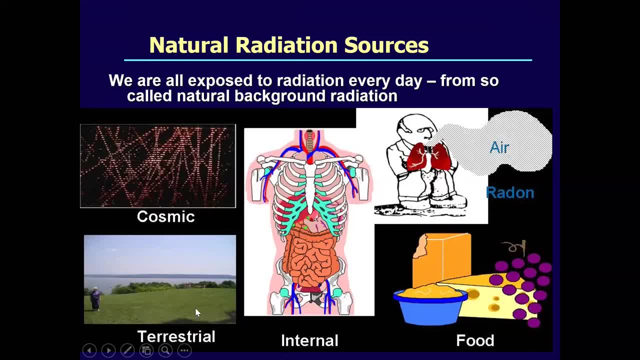 rocks which is there in the landscape, by which in those rocks there are highly radioactive isotopes, by which the thorium and potassium cerium, which are that naturally radioactive and their off life is their very large and it is always present there And these things, when we are consumed by food materials, we do consume a small amount of radiation, even. 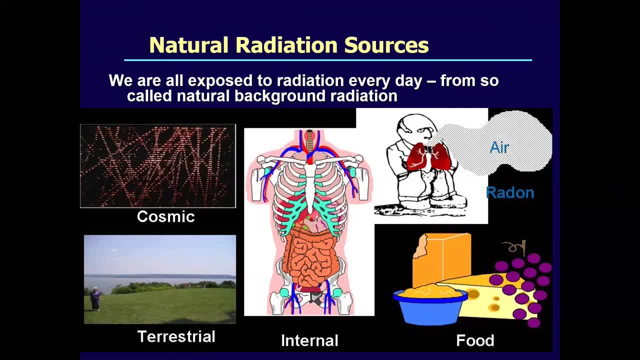 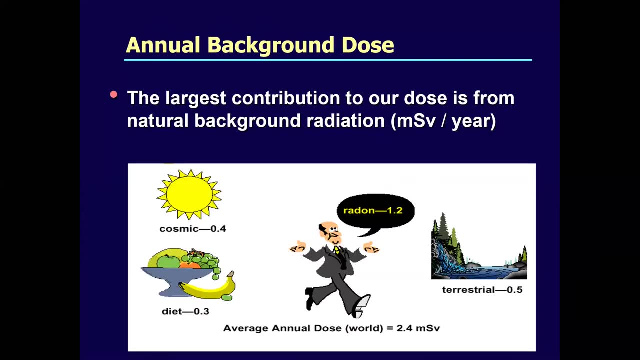 in the air. on, we have to. So the background radiation is invariably varying within a small ratio, Like, for example, if you look into the Kerala generally, the Kerala, the background radiations are slightly larger than the other parts of India. Now, in order to understand, they said: 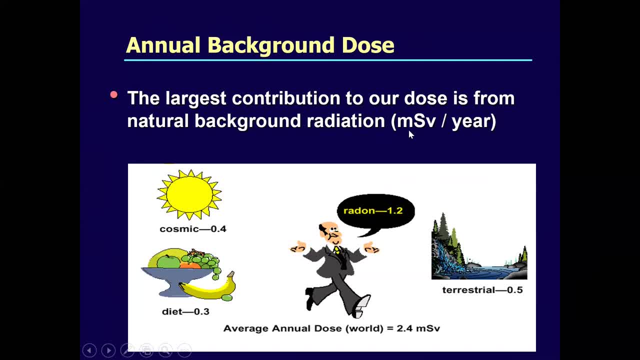 that the largest contribution of our dose is from the natural background radiation, which is expressed in terms of MSV. MSV stands for Millisievert per year And if you contribute the cosmic radiation is 0.4, and diet and other thing is 0.3 radon, what we inhale through. 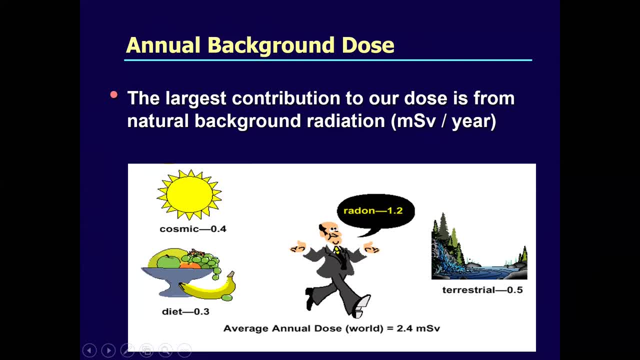 the air could be 1.2 times and terrestrial radiation is 0.5 and altogether accumulate an annual average dose, which means it's a global average ratio, which they say that all over the world. They look into the background radiation and made it a global average radiation dose, which 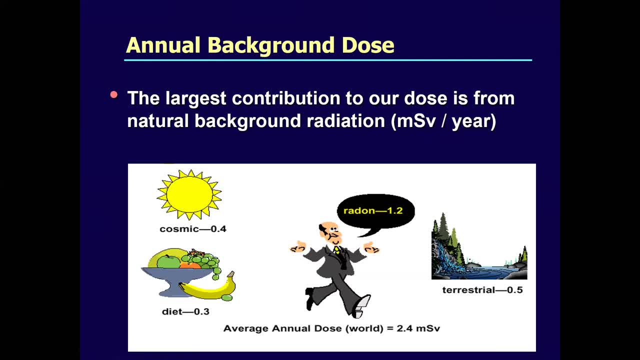 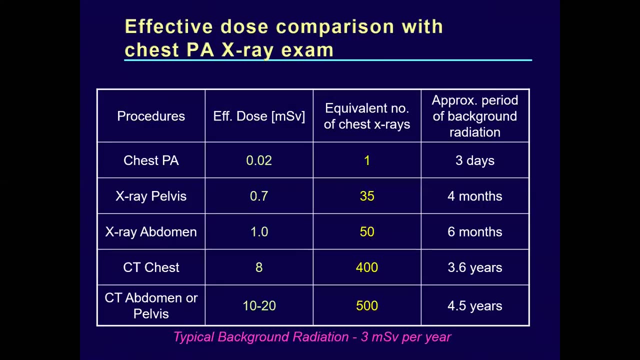 is 2.4 millisievert per year. So invariably, any parts of this globe we are there, a person may receive a radiation around 2.4 millisievert per year. So now let us ask the question: how does this background radiation compare with the chest X-ray or even the CT when we 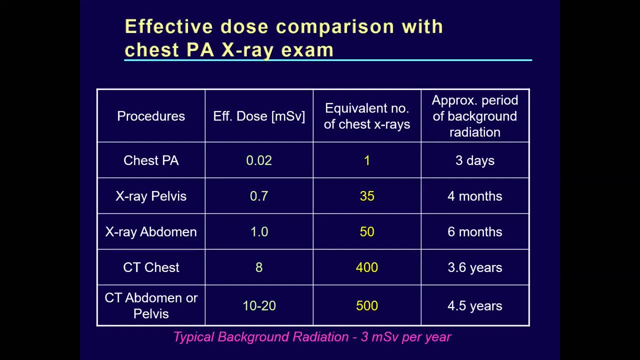 do for ultrasound? What are the diagnostic needs? So just look into the first, the chest X-ray. generally, I want to ask a question: Which, for an abdomen, in comparison to abdomen and a chest, which of the site will require more radiation? Is it the lung or the abdomen? It is the abdomen. 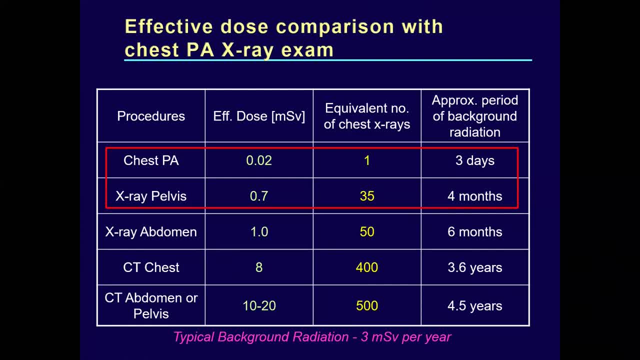 the chest Because it is the abdomen. The face is the abdomen, The chest is the abdomen. yeah, the chest has lung, where the lung density is much lower than the tissue density in our body. what is the atomic number of water? 7.4, and the tissue is close to water, so tissue has atomic 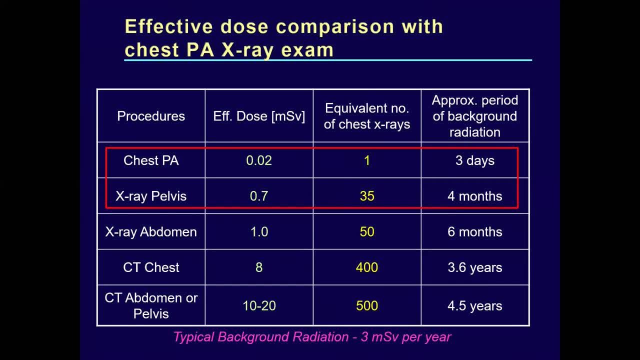 number of 7.42, whereas when it comes to lung, the atomic number is less and it the density is less. when you compare to bone, the bone density is 1.3 or 1.6 times higher than the soft tissue. so bones attenuate larger radiation compared to a tissue and the least radiation is by the lung. 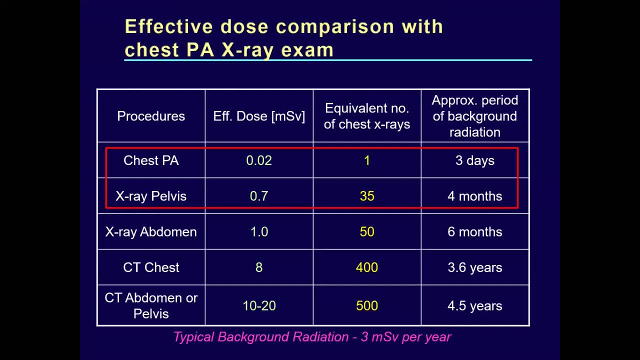 so when you want to take a chest x-ray, you give the minimum exposure in terms of. we call it as a. in order to give an exposure, we set a kv and ma. kv gives the penetrating power of the x-rays, whereas ma s tells the milliampere seconds of the current by which the x-ray exposure is going to be exposed. 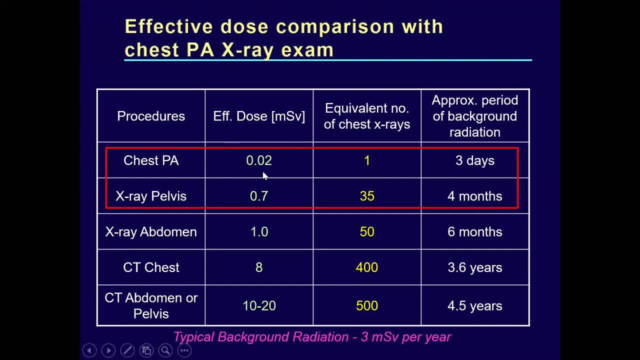 so for a chest x-ray when they give a very feeble radiation, it amounts to only 0.02 millisievert per year. if you roughly take three millisievert per year as the background radiation, this is just comparison of three days of a background radiation. that means by just doing a chest x-ray of a pa. 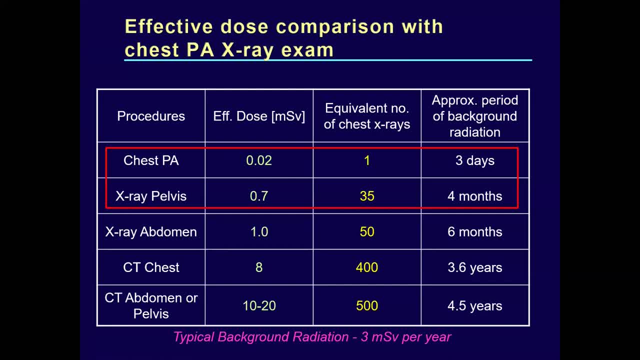 we are having a background equal to the background radiation of the x-ray. so the background radiation is very similar to a background radiation of three days, but the same thing when we do for an x-ray pelvis or abdomen. it is almost like a four months background radiation or six months. 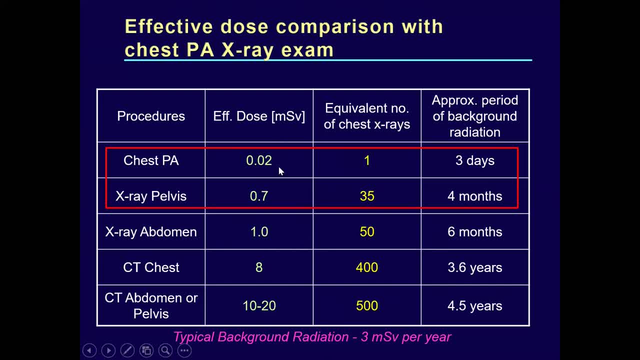 background radiation. so the 2d planar imaging requires very less dose and might be repeated often, depending upon the benefit of the patient, once you know it to have a diagnosis done. is it the same when we compare the plain or X-rays with a CT? No, 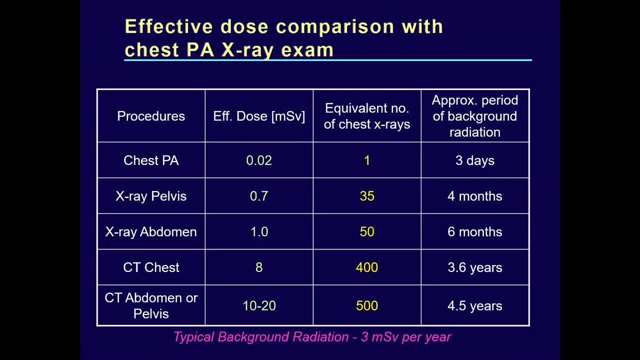 no sense. the CT dose received to a patient would be much larger in comparison to an X-ray. So before advising for a CT, you should always think whether a plain X-ray will do, or an ultrasound machine will do, or an MRI will do. Of course, an MRI is expensive, So many. 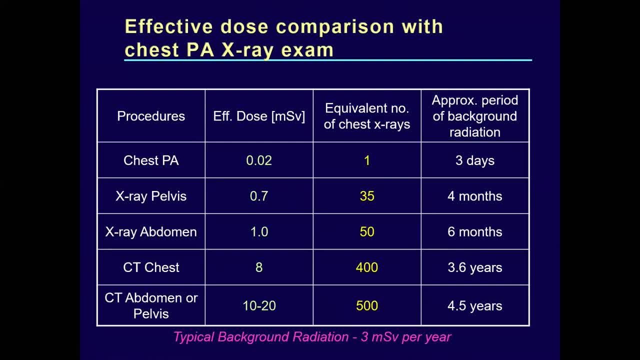 times. one has to also weigh the ratio of cost versus benefit as well. So when we take a chest X-ray, it is almost 3.6 times the background radiation, And when we see an abdomen, again it is 4 to 5.. So in a nutshell to say, a chest PA X-ray is very simple to be taken. It is. 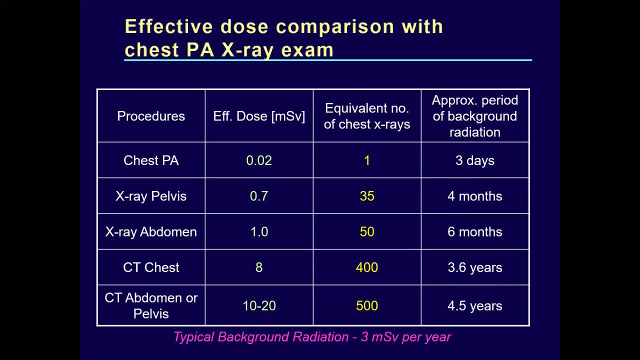 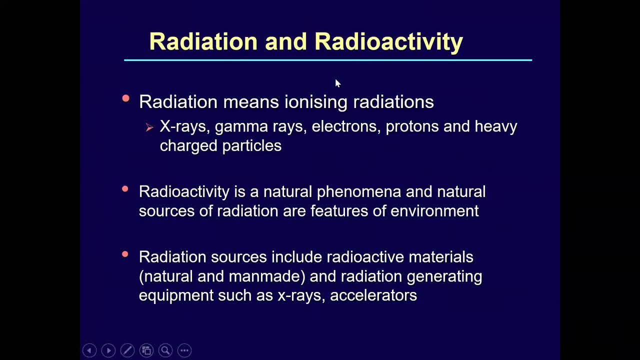 just like three days of a background radiation, And when you do volumetric imaging you have to think a little bit. Now, coming to radiation and radioactivity, What do we mean by radiation? Radiations are electromagnetic radiations And the spectrum includes X-rays, which is produced by an X-ray machine, gamma rays. 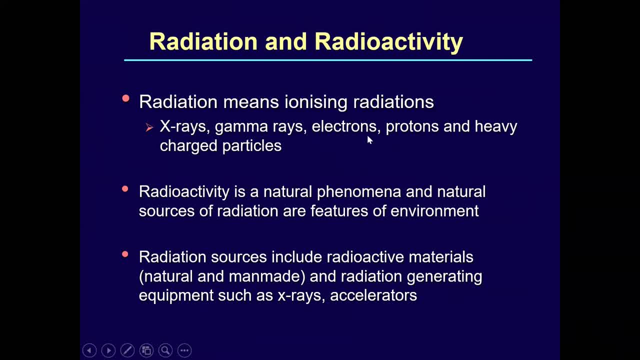 which is produced by radioactive materials. Electrons again can be produced by the X-ray machines, And protons and heavy charged particles are produced on accelerators and research centers. Radioactivity is a natural phenomenon. The disadvantage of radioactivity is that 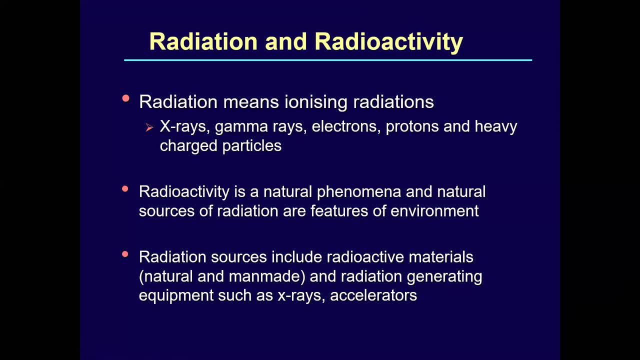 we all have learned in our schooling center: radioactivity will always decay depending upon the parent product to the daughter And its half-life will be always. After one half-life the radiation decreases to 50% of the intensity. Then again the next half-life, another 50% In order to have a significantly 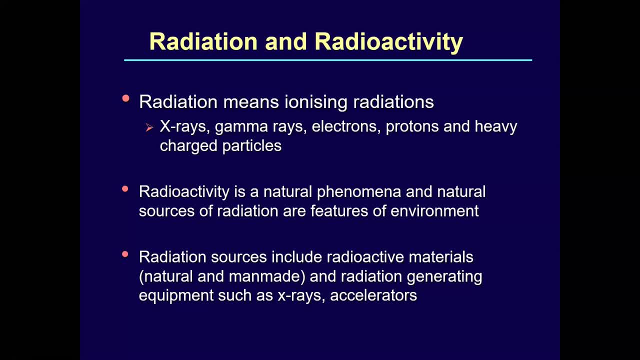 negligible radiation. you have to minimum have 4 to 5 half-lives for normal radioactive isotopes. But when you consider cobalt-60 or radium or cesium, which are heavily used for radiotherapy purposes or industrial radiography, They need to be used for the purpose of reducing. the degree of radiation which is very common in radioactivity. Because of this, there is a lot of difference. Now we will see this through radiation, So we have to see the solar radiation, which is very weak in charge of radiation, And if you have a πολύ high radiation level, On the other hand, 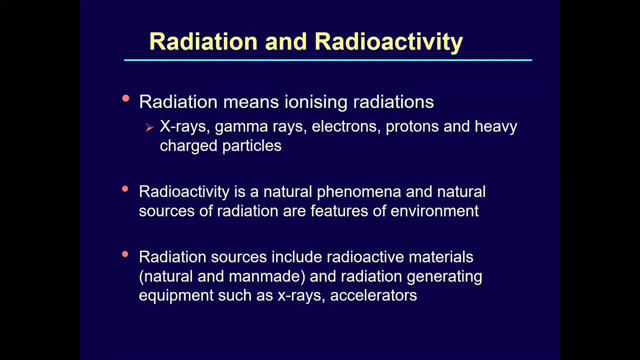 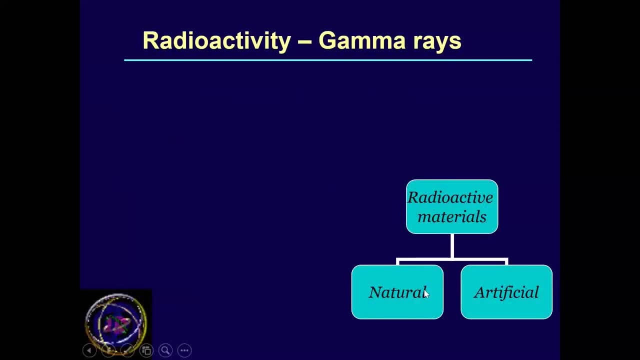 even kept on for a very long off-life and disposed very appropriately, otherwise it can be a potentially a very harmful thing. so radiation can be from natural as well as artificial, artificial means. we are going to use the reactors in the baba atomic research center or kota rajasthan. 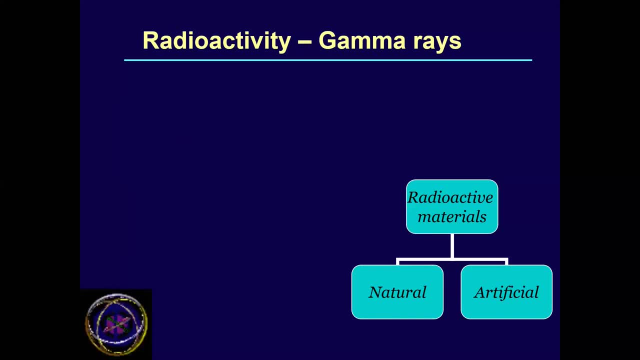 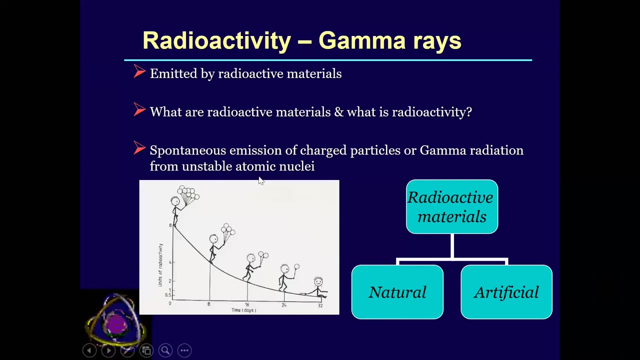 where they bombard on a neutron environment, a cobalt source, and then make it radioactive, so that radioactivity, once it achieves the radioactivity it keeps spontaneously emission of charged particles, either gamma, alpha, beta, to begin into a stable atom. now look into this diagram. i would like to have your attention. first look into this thing: a radioactivity. 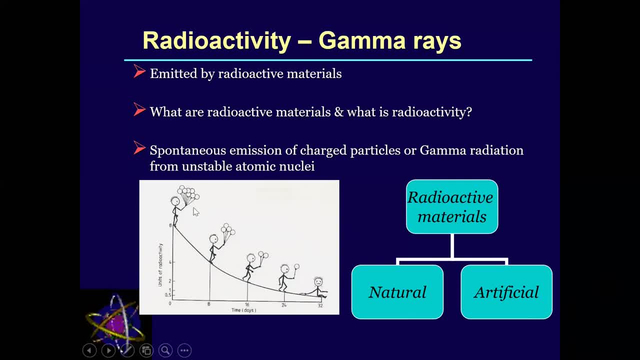 the initially when, at a given point, there are eight balloons here, okay- telling that the radiation in intensity is 8 units and the half-life is 8 days. So after 8 days the intensity has decreased to 4 units, and after next 8 days- 16, it is decreased to 2. Then another 8 days. 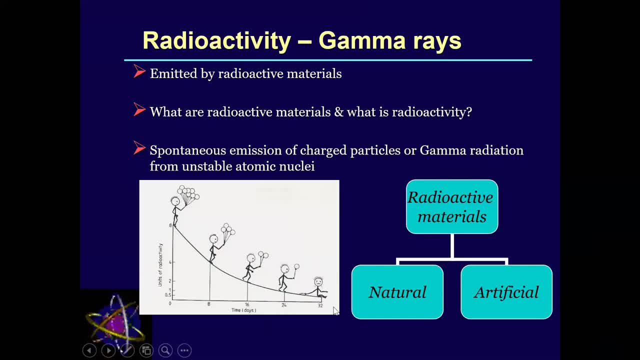 which is 24, decreased to 1. Then another 8 days it decreased to half unit and then quarter unit. So it keeps exponentially going. That's what I said Generally. a radioactive isotope kept over a long period will reduce its intensity and when it achieves insignificance. 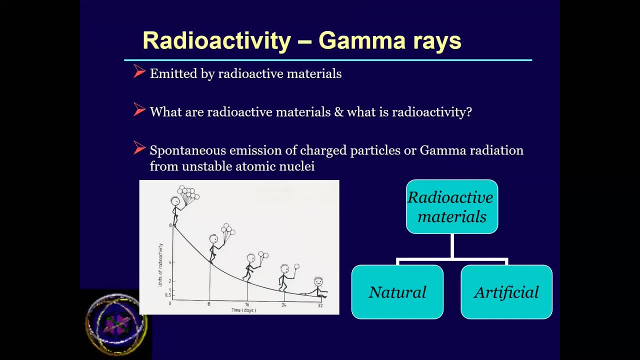 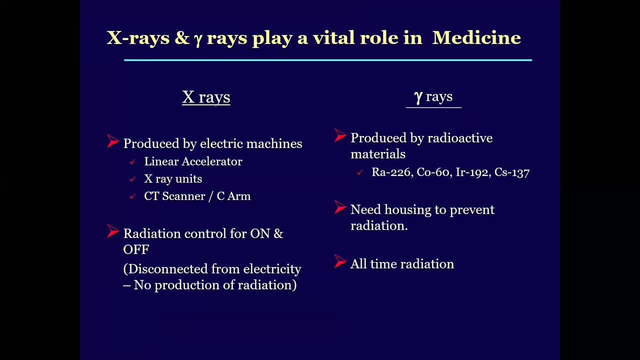 then it has been not discarded Again. it is safely disposed, because we need to have a safe disposal practice and that is a mandate. So what is the disadvantage between radioactive isotope comparison to X-rays? X-rays are produced on electrical machines like linear accelerators. 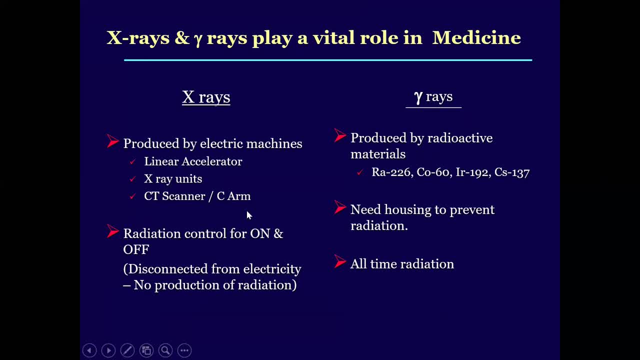 X-ray units, CT scanners or a CR machine, Whereas radioactive materials are produced either natural or artificial, like iridium-192 is an artificial radioactive one used for brachytherapy, Radium and cobalt. they are used for external radiotherapies and they need to be housed in a proper environment. 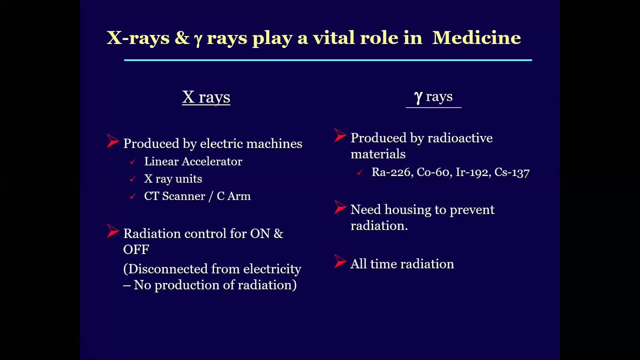 with a high atomic number, housing material to reduce the radiation from other directions and only in one direction. In one direction there is a collimation and by a radiation switch on, switch off mechanism you can make the radiation on, use it and make it off. Remember the background radiation. 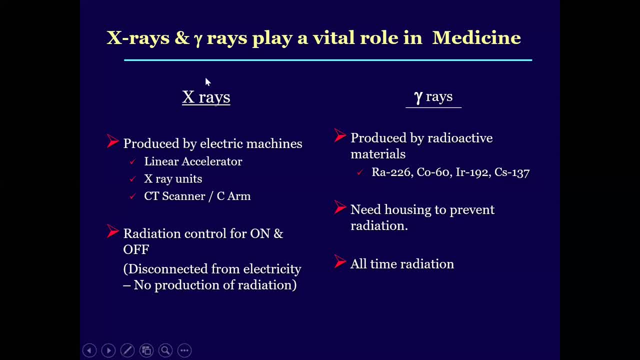 or the leakage. radiation is always present here When we come to the X-ray units. as soon as we switch off the electrical power, there is no radiation. So the radiation is only on when we want to keep it on, use it on the electricity and then switch it off. 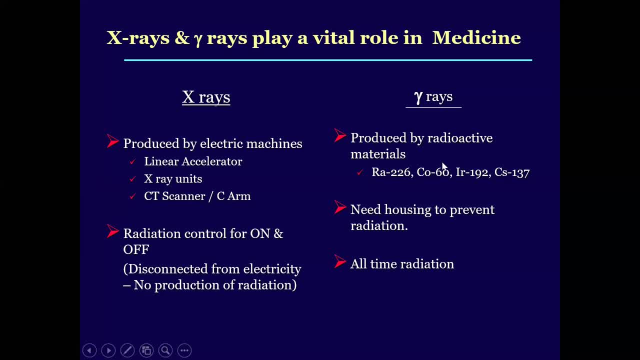 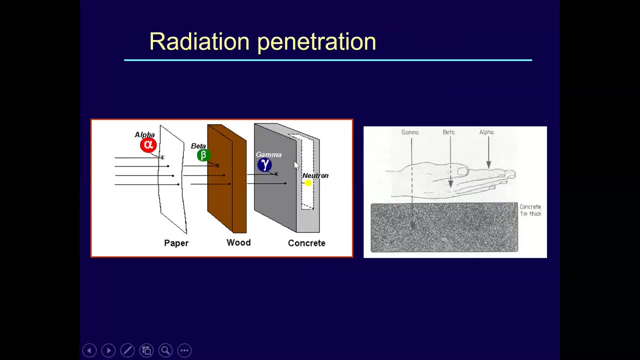 So this says that yes, using a radioactive isotopes is more. you need to have a very healthy practice and a safe practice, and periodic quality assurance is our mandate. Now I talked about Alpha Beta, Gamma radiation, and we should also know Alpha Beta is a very heavy 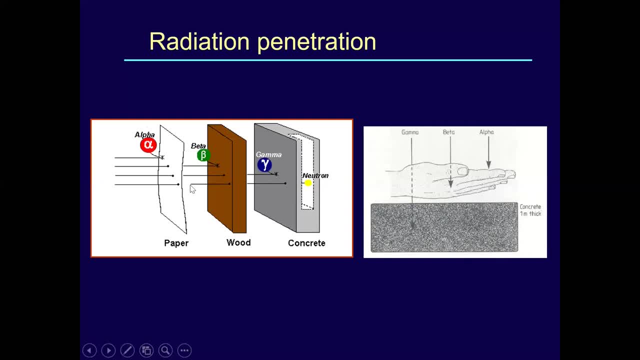 charged particle and its transmission will be very less that it can be even attenuated by a piece of paper. But the radiation damage is different. In the subsequent slide I will talk about the radiation biological effect of different radiation. Here you only understand, since alpha particles 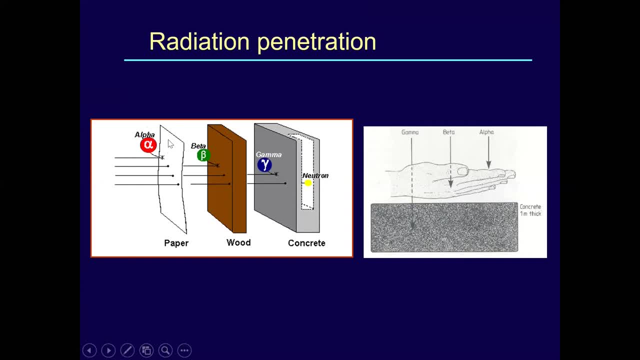 are heavily charged and their particle size is larger. they can be attenuated by a piece of paper, Whereas beta particles or electrons they can traverse through a wood or a tissue very easily. But they can be attenuated very easily by lead or concrete. When we come to 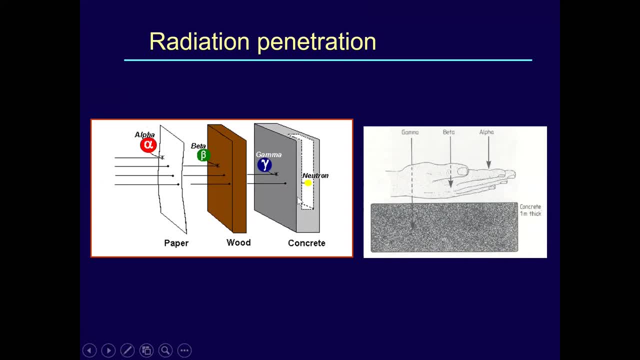 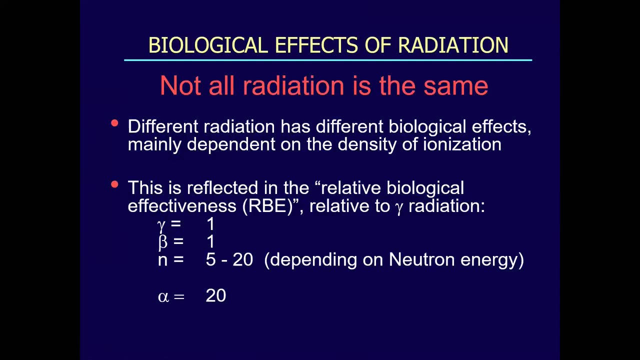 neutron particles or gamma radiations. even if you have a heavy, concrete still, the radiation can transmit. only its intensity reduces, but the transmission of adequate radiation will be always happening. Is that clear? So now I again talk about it. These three types of 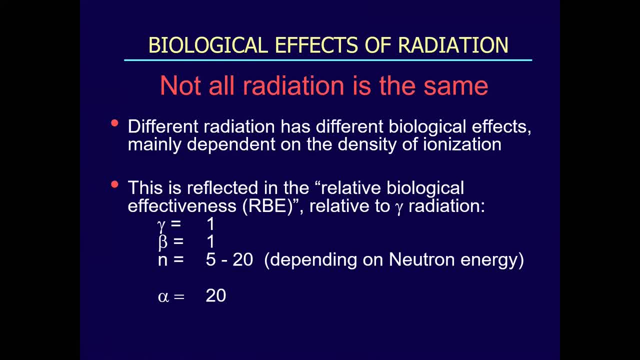 radiation- Alpha, beta, gamma. What is the radiation effect? What is the radiation damage they can do on the tissue? The alpha particle will have a heavy radiation damage like 20 times. We equate the gamma or the X-rays as relative biological effectiveness, RBE. So the RBE is 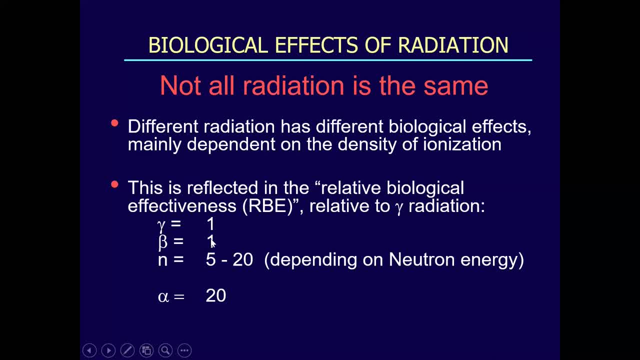 one for gamma and X-rays, As well as beta and electrons. But when it comes to thermal neutrons, depending upon the neutron energy, whether it's a thermal or it's a heavy neutron charged particle- the RBE ranges from 5 to 20,, which means a dose of 100 units given by a X-ray machine. 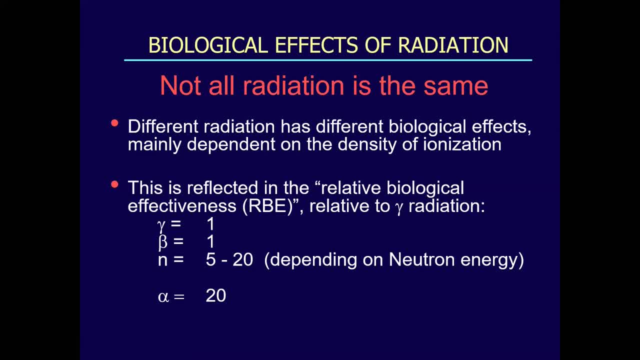 will produce only 100 units of damage, Whereas if it is a neutron it can be 100, into 20,, 2000 times the damage. The same thing is true with the alpha particle, So the beta electron is given. So if a same dose is given by different type of radiation, the damages can be different. 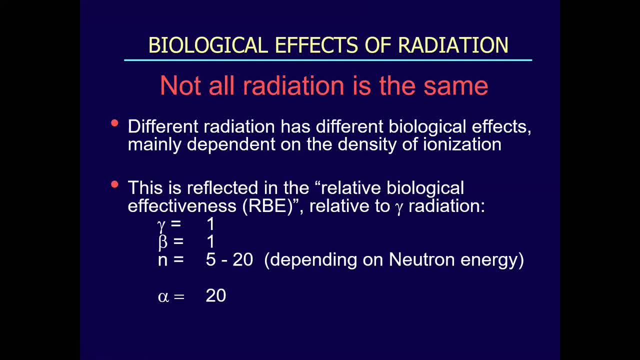 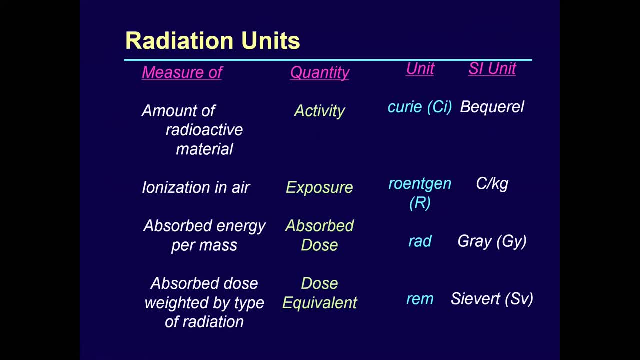 In a similar way, the sites also, the body sites also have a different sensitivity to radiation. So now let me talk about radiation units. So when we talk about radiation units, radioactivity is called in the name of activity. Curie Si unit is becquerel when it ionizes in the exposure form When we are giving exposure. 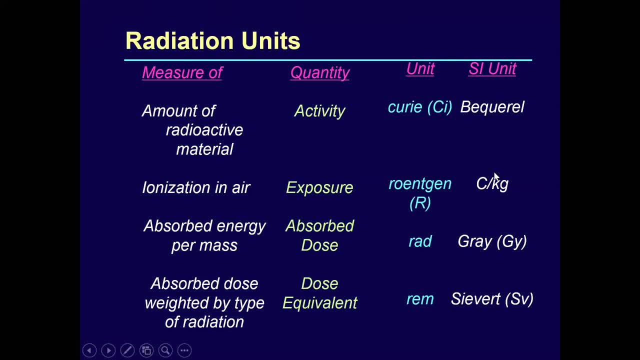 to a patient. we call it Rongen and the Si unit is coulombs per kg. In radiotherapy, when we wanted and we are interested in the absorption of radiation dose, we call it as the rad Rongen absorbed dose. Rongen absorbed dose is rad, short form and the Si unit is gray Wenn we. 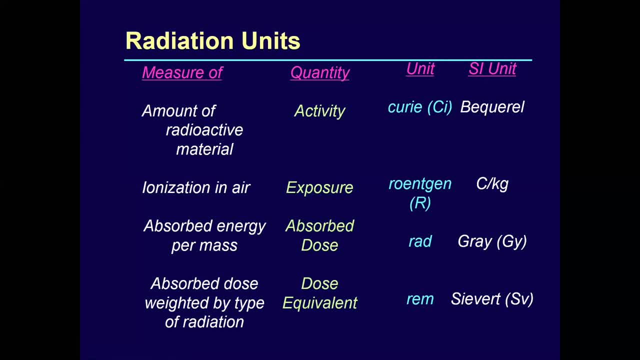 radiation protection. As I told you, different type of radiation can have different damages, as well as different sites like the gonads and the embryos, and the islands can have a different sensitivity for radiation. So we need a radiation equivalent dose, which is called radiation equivalent rem, And its SI unit is Sievert. Also remember Sievert milli. 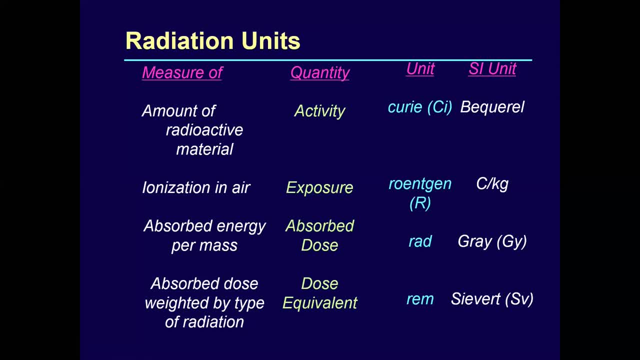 Sievert means 10 to the power minus 3.. Micro Sievert means 10 to the power minus 6.. As we put Sievert, it is a larger unit, Milli Sievert, 10 to the power minus 3 and micro. 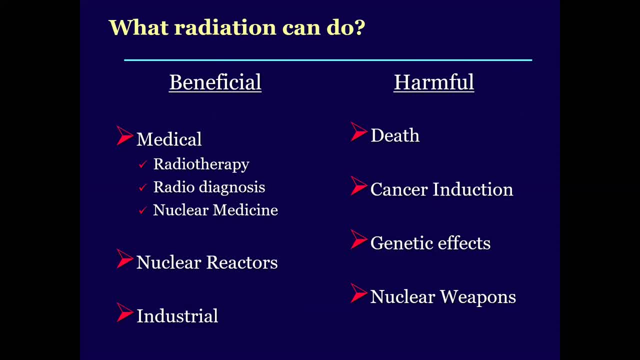 10 to the power minus 6.. Ok, now what radiation can do. Can radiation be beneficial? Yes, it is certainly beneficial if we use it in the right way and right practice. It has been proved to be useful In clinical practice for a long time, either radio diagnosis or radiotherapy or nuclear. 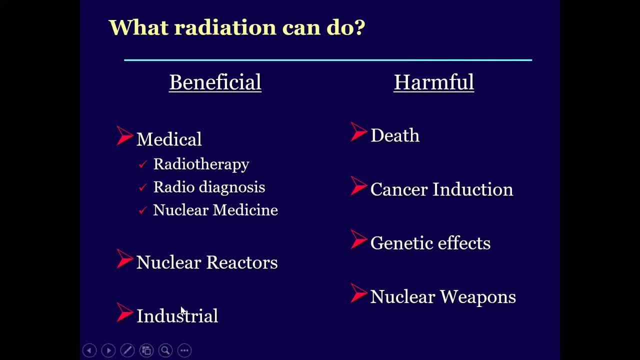 medicine, for the matter, For nuclear medicine. we use it for imaging as well as therapeutic Nuclear reactors to produce so many radio isotopes for industrial testing and many other things for industrial purposes, But at the same time, when the radiation is mishandled, 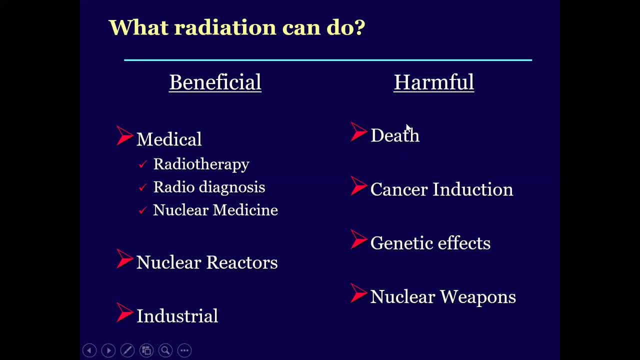 and if you give a large amount of radiation to a person it can even have the event of death. The other one is cancer induction. So cancer induced secondary cancers can be produced on a patient. Genetic effects. Even a patient who is being exposed to radiation may have 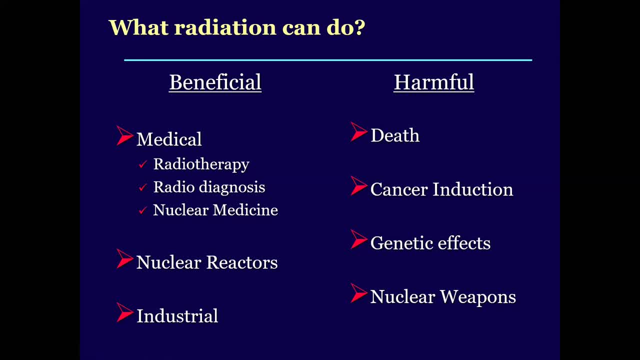 their generations, one of the second offspring to have a breast cancer. So that is possible. Then again, if it has been used in the wrong direction, it can be used as a nuclear weapons. Now, this the reason. then again, this is not because theprechen of radiation is wrong. 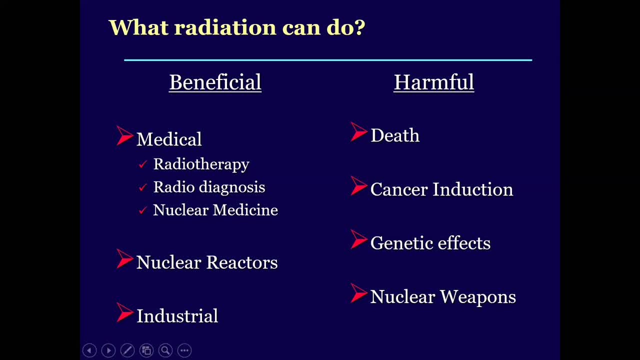 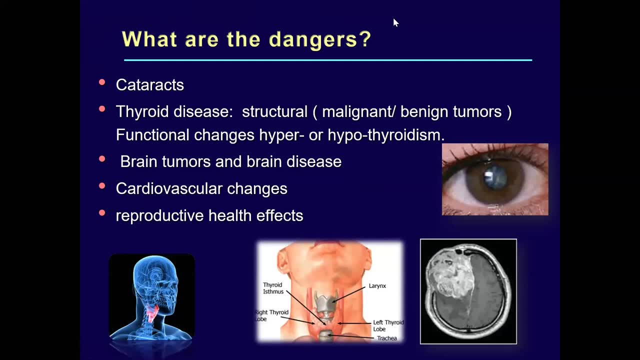 But we see that this is the increasing of radiation. In the case of radiation we cannot as a nuclear bombs to damage and produce harm. So what are the biological damage of radiation? Biological damage of radiation is that radiation can produce you cataract. It can have thyroid. 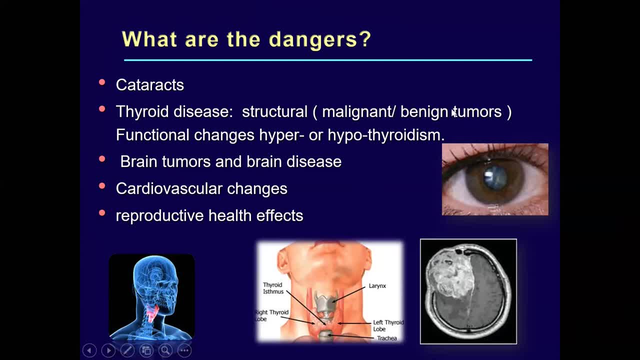 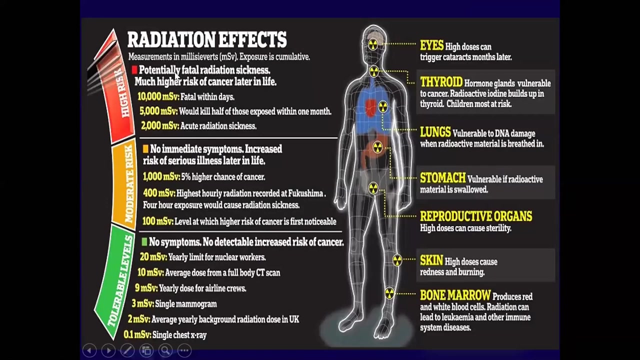 radiation to the thyroid can be malignant tumors or benign tumors. It can manipulate the functional characteristics of the thyroid. It can have a brain tumor. It can produce cardiovascular changes and also reproductive changes. So here look into this slide about the radiation effects. 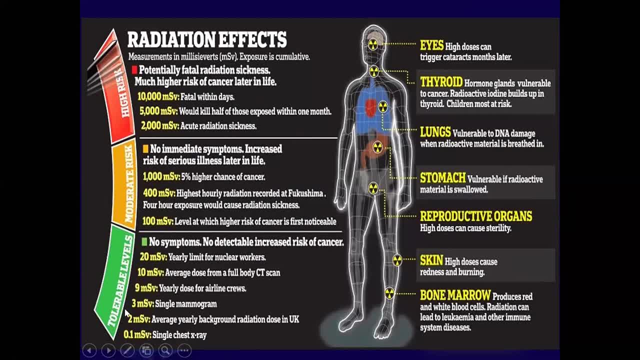 The lower one, which is this green, is the tolerance level. Now, do you remember what was the average background radiation? It is 3 millisievert per year. The 3 millisievert per year is equivalent to a single mammoth When we do screening process for a females. a single mammogram will give you a dose of 3. 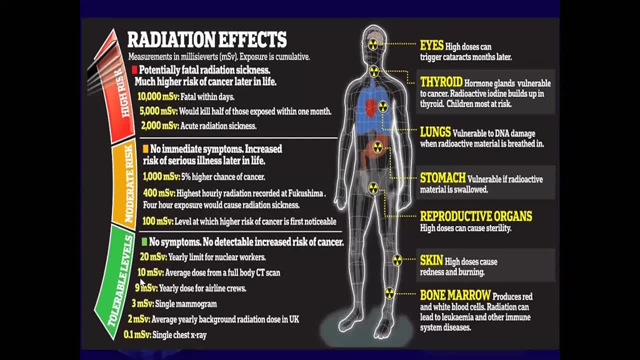 millisievert. So up to radiation of 20 millisievert is considered to be very, very least and tolerable and in fact there is no symptom or no deductible increased risk of cancer. So that is why 20 millisievert is the average. So up to radiation of 20 millisievert is considered to be very, very. 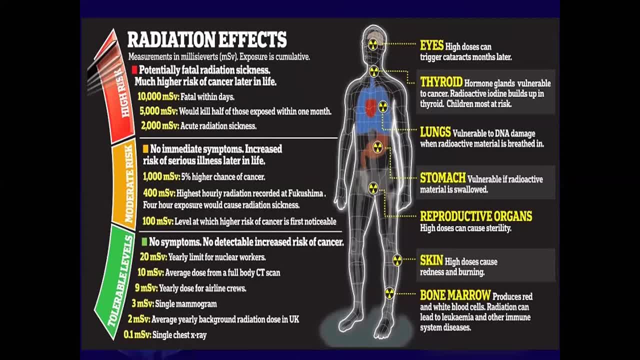 less than 2 millisievert in factor, The upper dose limit for any radiation workers. You might have seen lot of radiation employees wearing a small film badge on the chest So that badges keeps monitoring the radiation and their upper limit per year they can have is only 20 millisievert. 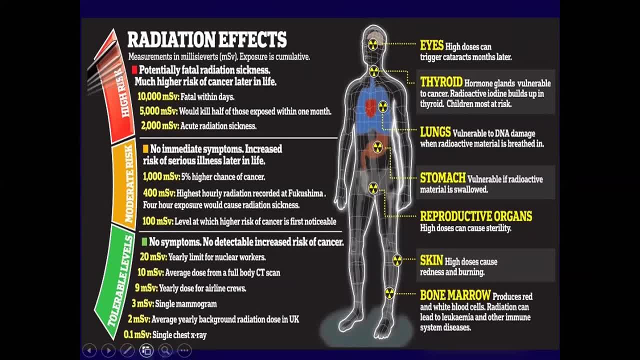 So here, for any investigation purposes, when we do the single chest X-ray to a whole body, CT, this X-ray will not give high risk mortality. So in the absence of any x-rays, any x-rays can be carried to the chest, x-ray to a chest. 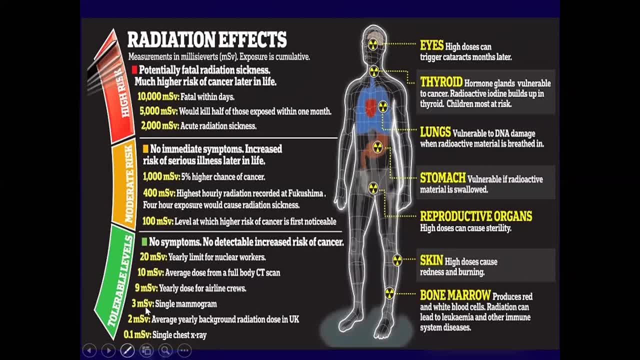 x-ray to a whole body CT. So with this, if it is no complication, then it is normal live body CT which is 10 millisievert we can do, which is very safe practice. Then comes the moderate, from 100 millisievert to 1000 millisievert. Generally this kind of a radiation is never. 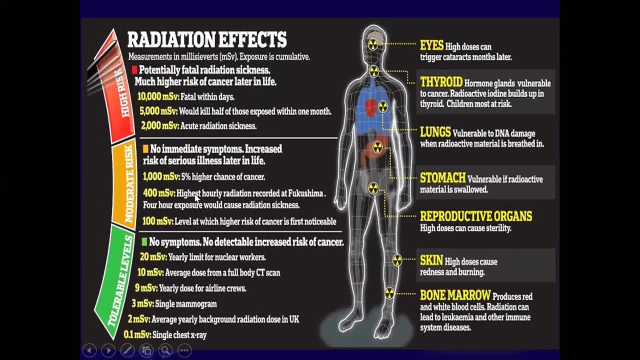 encountered, unless until there is a radiation accident or an X-ray tube which has been repaired in a wrong way and the shielding was not placed properly, or radioisotope has been left open, or, in the nuclear medicine, the radioisotope has been contaminated on the clothes and the clothes. 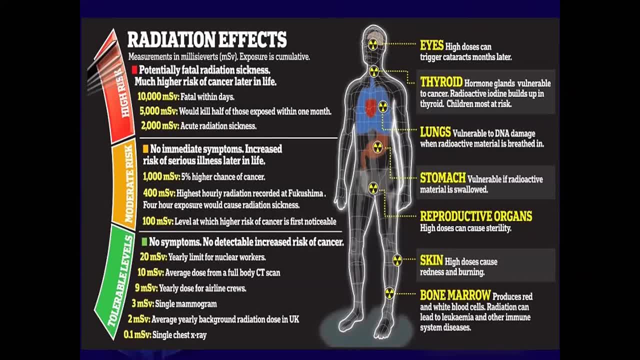 you have been wearing the apron which has been contaminated with the radioisotope, So or it has been a radiation bomb in like a Hiroshima, Nagasaki, Bombay, sorry Japan. So I say bomb blast. may the background radiations keep giving at places and some places, if. 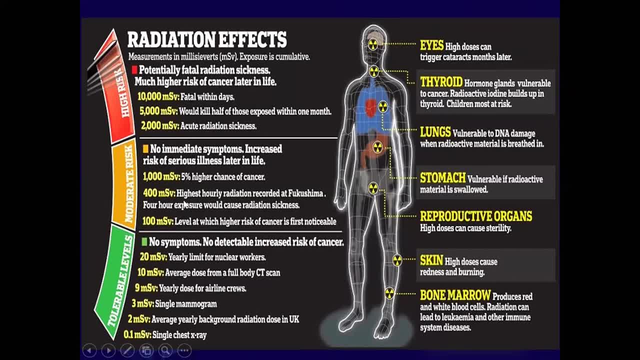 people are start living, they do get moderate amount of doses, which is a risk production. So this radiations is considered to be risk and even in this, depending upon the amount of radiation, they will have certain symptoms Beyond this, like 2000 millisievert, if you have a radiation it is a very high risk. 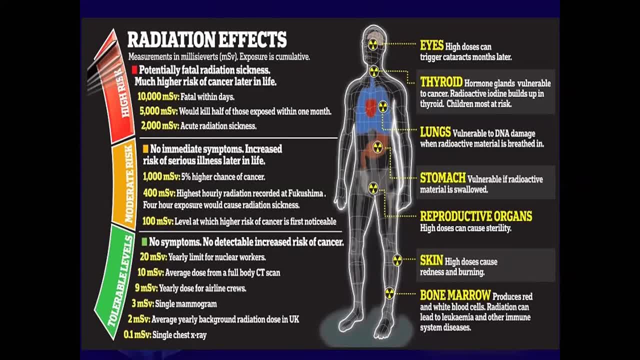 and it can produce acute radiation sickness. So this is the symptom: when you have an acute radiation sickness, that means you have been consumed to a very large radiation exposure because it affects the bone marrow, you have skin reddening producing and burning comes and you produce a lot of biological damage. 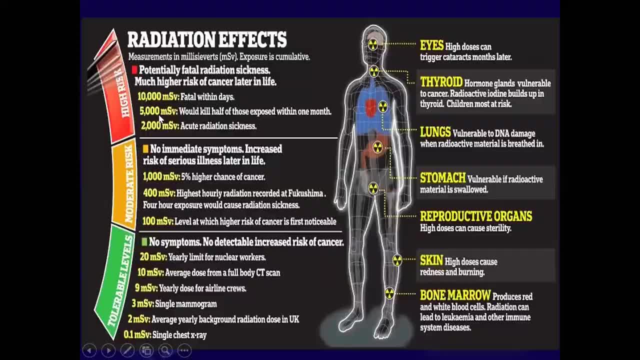 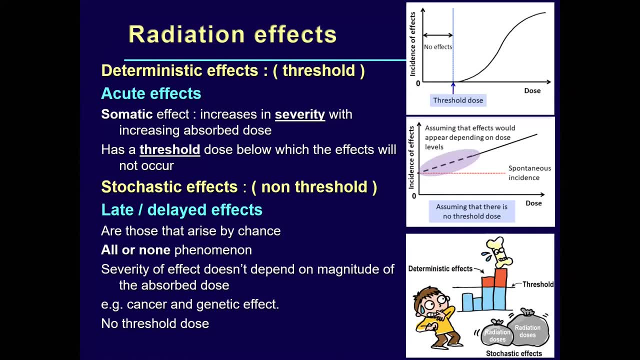 in this high risk region. So now coming to radiation effects, there are two types of radiation effects. One effect is deterministic effect. Deterministic effect means there is a threshold. You see this curve. it has a sigmoidal curve And you have a threshold value and you can set a threshold value on the sigmoidal curve. 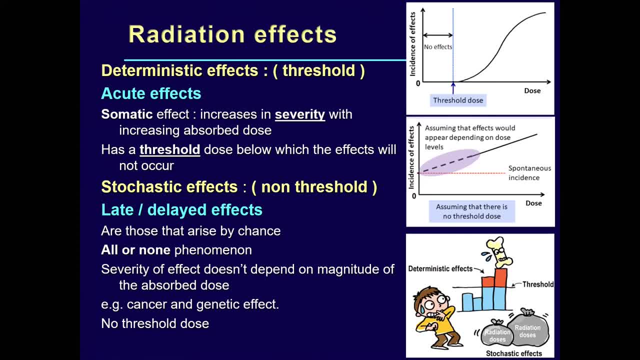 and say below this threshold dose there is no significant radiation effect. Beyond that there can be a radiation effect and the severity may increase with the increase in dose. So beyond this particular, as you increase in the dose the severity of the effect may increase, the incidence probability may increase. So this is the deterministic effect. 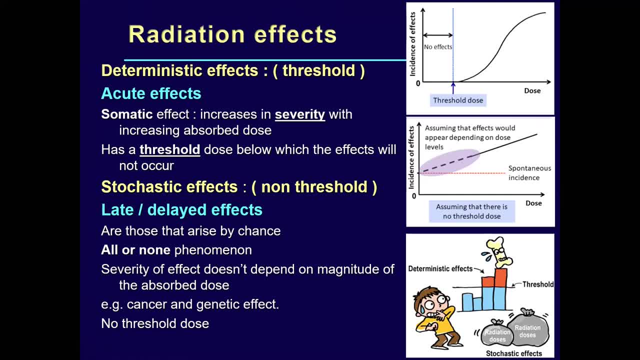 So for deterministic effect. since we know the threshold dose, we can tell 500 centigrade is a limit for the lens and beyond which the lens gets a dose a cataract may be formed. So either we can avoid it if we know the limit, or if the lens is damaged you can replace it. 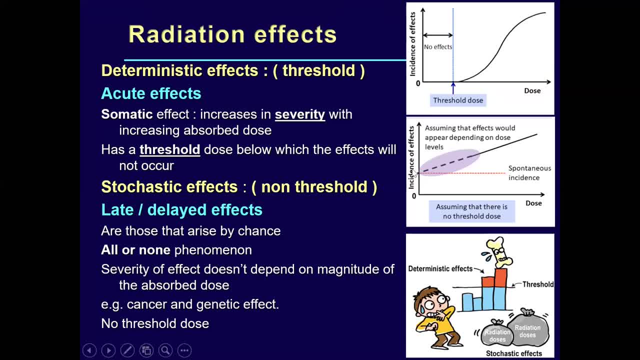 Now, if you come to the other effect, which is called stochastic effect, this doesn't have a threshold. So we don't know what is the threshold dose. So even a small dose can have a possibility of a radiation, and it could be all or none if 10. 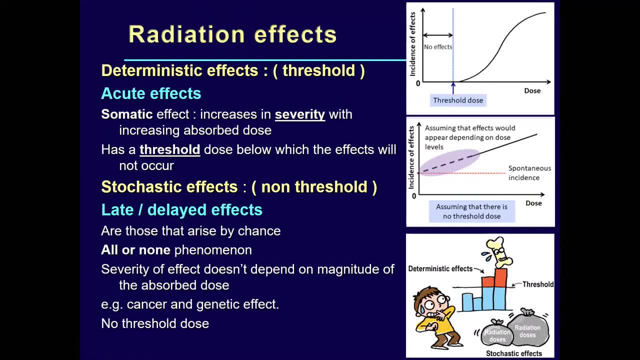 group of 10 persons have been irradiated. sometimes even all the 10 may get a radiation damage, or only one may get a damage. So similarly, there is no. the increase in dose will not increase the severity that much, So it is very difficult to account for this. That is why. 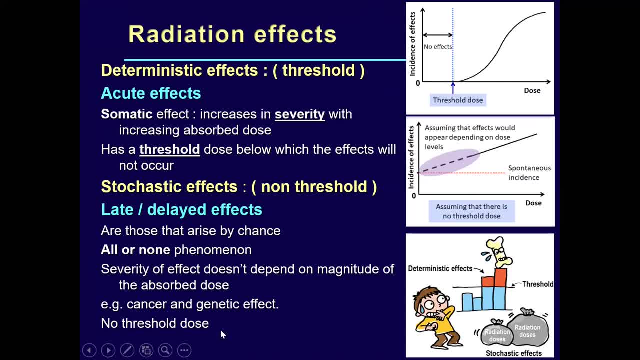 there is no threshold, So we have to avoid as low as dose possible. There is one more word, a key word. what is used in in radiation protection is ALARA- as low as radiation achievable. That means either when you are working as a radiation worker or for radiation dose to patient. 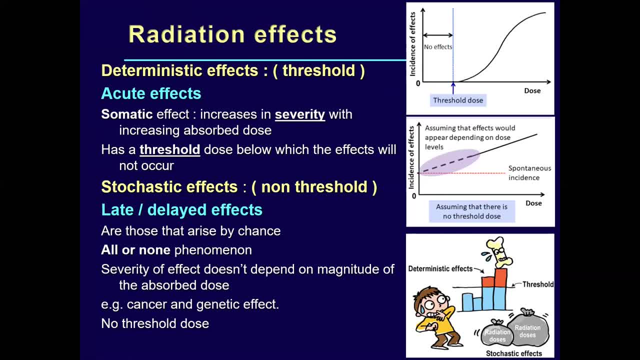 you have to always do as low as dose Because we know no radiation is safe To have. prevent deterministic effect we can do because we know the threshold. we can prevent a radiation induced cataract but a leukemia, a blood cancer which is a caused due to the radiation we cannot prevent. 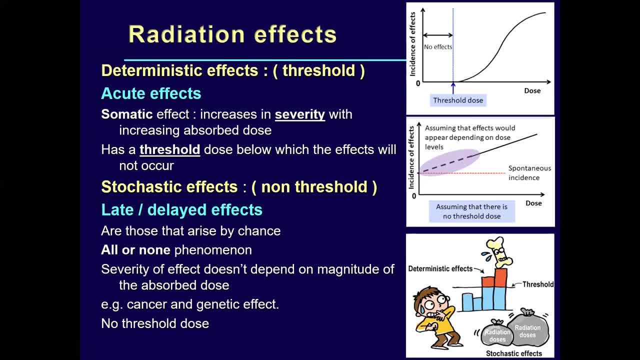 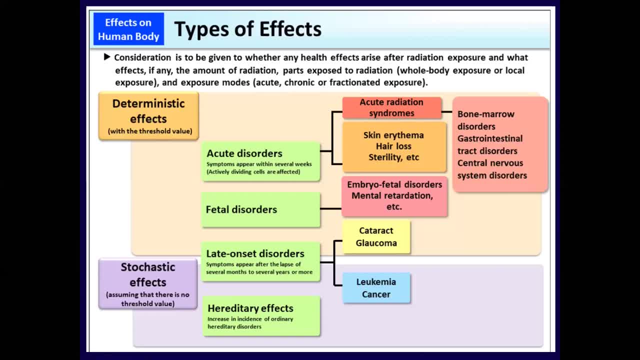 So we have to always stay out of radiation and we could, we can only recommend as low as possible of radiation. So I am summarizing the same thing: Deterministic effect we can avoid if we have a safe practice. Stochastic effect we cannot avoid because there is no threshold. So we have to follow the principle. 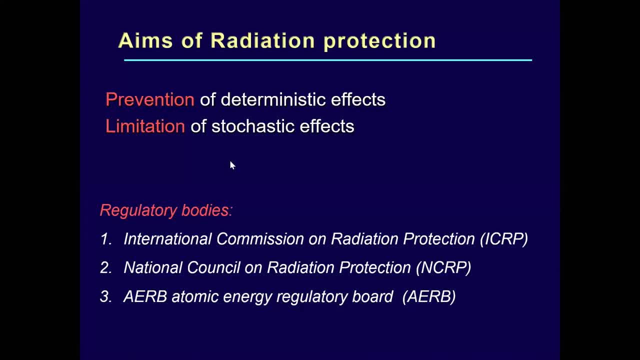 of ALARA as low as reasonably achievable. So the aim of radiation protection is to the prevention of the deterministic effect and limit the stochastic effect. because we cannot eliminate the stochastic effect And there are international bodies like International Commission of Radiation Protection, ICRP, and National Council of Radiation Protection, NCRP, which gives guidelines. 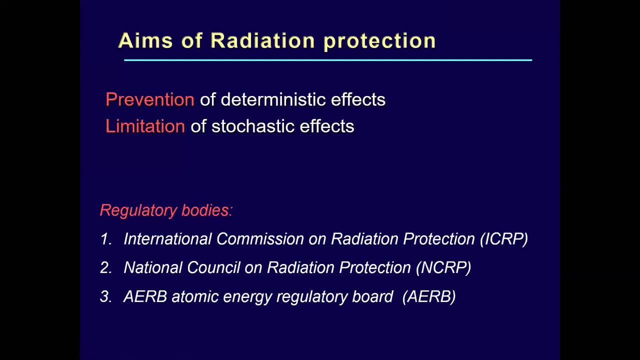 and radiation safety stipulations across the globe, for the world. For India, there is an Atomic Energy Regulatory Board which again stipulates the guidelines to be practiced in our country, and they are the authority for us to give licensing, and licensing for operation of X-Ray equipment. 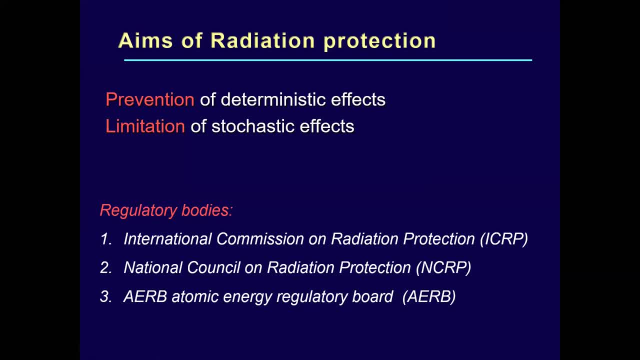 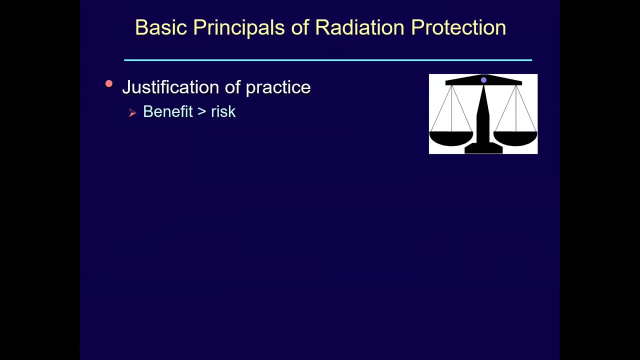 and monitoring of radiation safety purposes for India. So what are the principles of radiation protection? Principles of radiation protection are always benefit versus risk. So always the benefit should be larger than the risk. Doing a chest X-Ray is not at all a big risk. Doing a 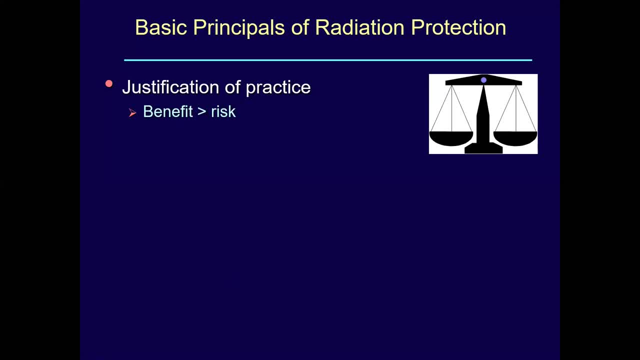 Doing an abdomen CT is a small risk, but again you need three-dimensional data and you are going to do a surgery. You want to know what are the organs inside and how the disease is going on, or what are the organs you need to remove, what are the adjacent structures. 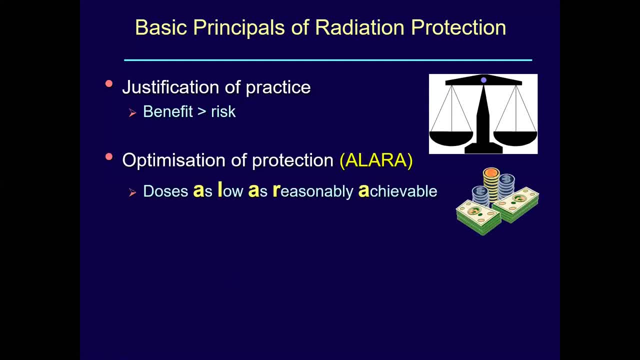 You may have to see it three-dimensionally, So you need it. So, as I told you, optimization of radiation is very important for protection, which is ALARA doses as low as reasonably achievable. Now, as I told you, deterministic effect: there is a threshold dose. 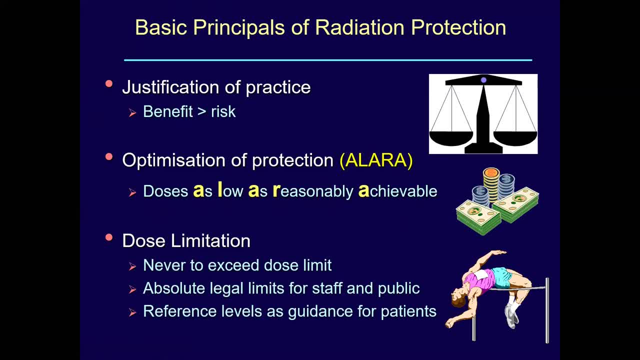 So when there is a threshold dose, always go and limit by the threshold dose And also for radiation protection for the staff. if 20 millisieverts is the higher limit, we have to respect that. beyond 20 millisieverts they are not supposed to be exposed. 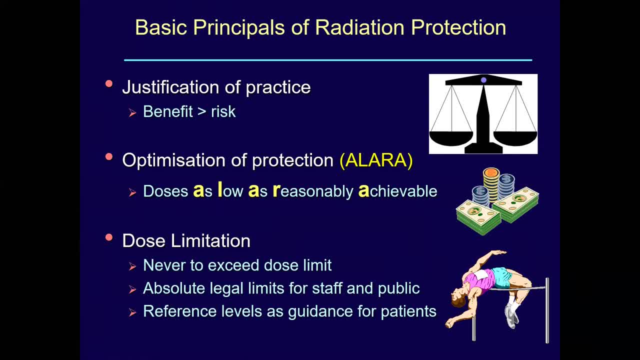 And if they are exposed during the quarterly radiation measurements, we have to do investigations to measure. So again, there are radiation legal limits Below 18 years of age. you cannot employ a person, even as a trainee. they cannot be. 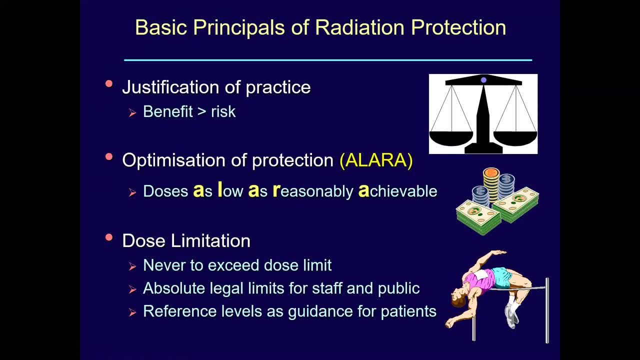 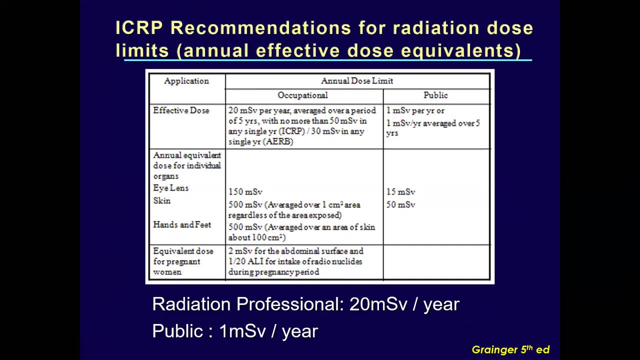 trainees who can learn radiation like x-ray technicians. They cannot be below the age of 18.. So what is the ICRP? recommended doses for annual dose limits: Okay, The effective dose limit should be 20 millisieverts, averaged over a period of five years. 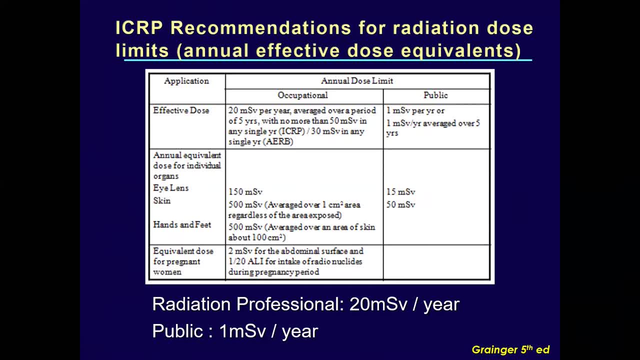 What does this mean? You can take 20 millisieverts per year, but it doesn't matter if it is 30 millisieverts in any year. Over a period of five years, you should get an average of 20 millisieverts, and in a particular 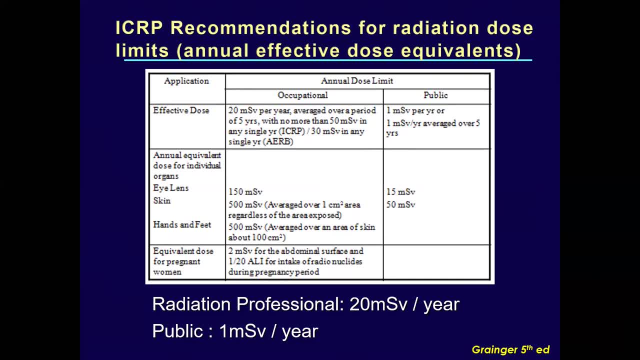 year you can get up to 30 millisieverts And this is for radiation workers. When you come to the general public, only 1 millisievert per year. Okay, But we should not include the medical exposure, what they do for the benefit of diagnosis. 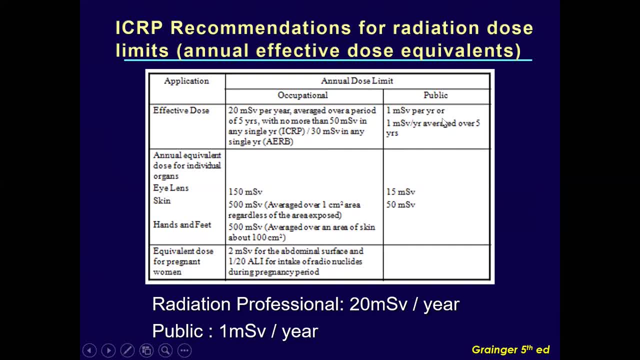 or therapy into this. radiation doses, Same with the radiation workers also. Any medical radiations, whatever we do, is not accounted into it. Like, for example, any radiation worker is undergoing a CT, he should not wear a film badge. So now come to we should know the radiation dose limits for the pregnant female also. 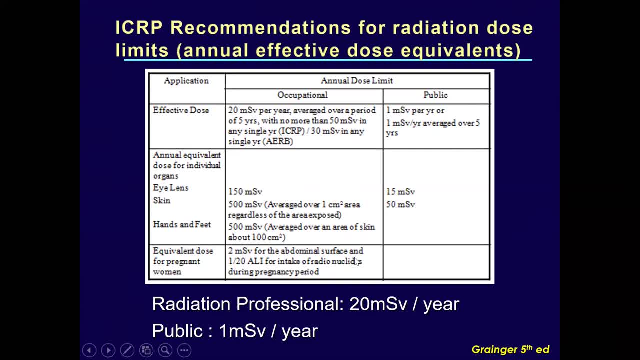 Okay, So 2 millisieverts for the abdominal surface for the entire term of pregnancy. or if it is a nuclear medicine, radioisotopes in yield 1- 20th of the annual dose limit. it should be within 1 by 20th. 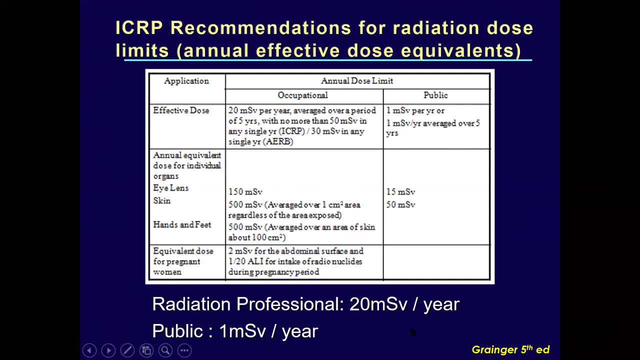 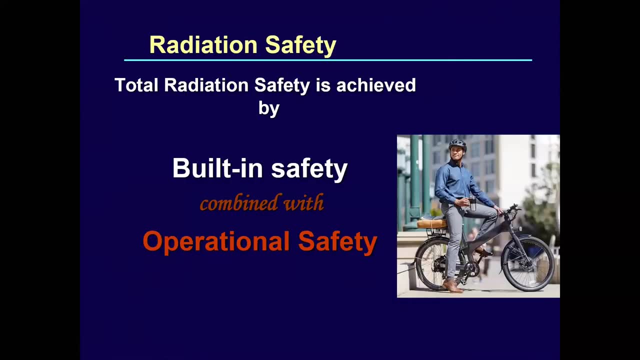 So, in order to keep in memory, 20 millisieverts per year is the radiation dose which a radiation worker can receive. General public will receive 1, 20th of it, which is 1 millisievert per year. Okay, Now, like any other thing, any other safety- fire safety or biomedical based safety- radiation. 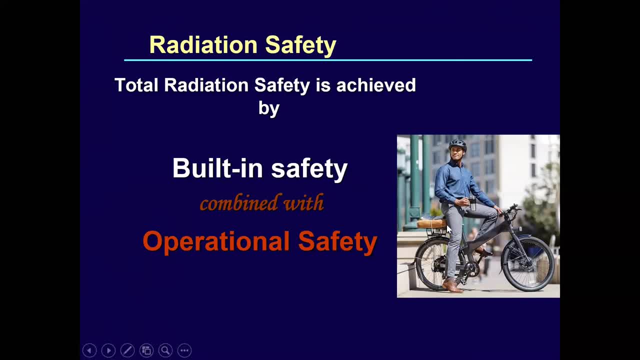 safety also has its functional built-in safety. All radiation working environment and equipments have operational safety. So we have to combine the operational safety of the equipment, how it is designed, with the built-in principles of the functional physical safety. Okay, Thank you. 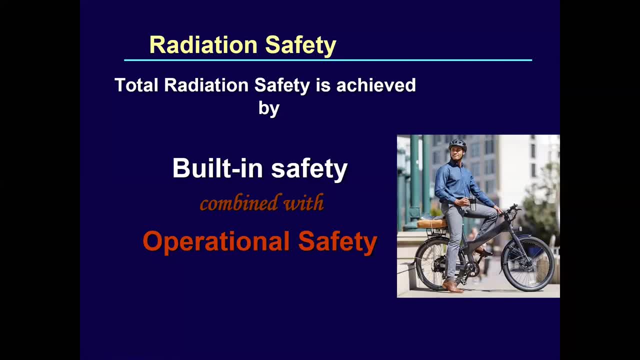 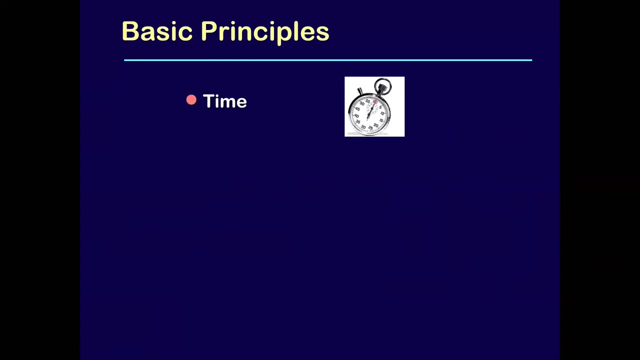 So equipment, how it has been designed and how it has been operated. both are important. Like a cycle may be well designed with the brakes, but of course the operator should know when he has to apply the brakes For that in radiation protection. the three important things, what we look into, the thing. 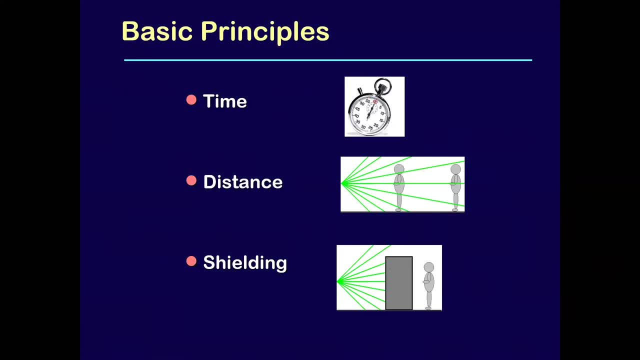 is that time? distance shielding. Time means the minimum time we should give. Minimum time we should give exposure so that the radiation is not given for a long over. exposure wherever it matters. and distance, if we increase the distance instead of standing. 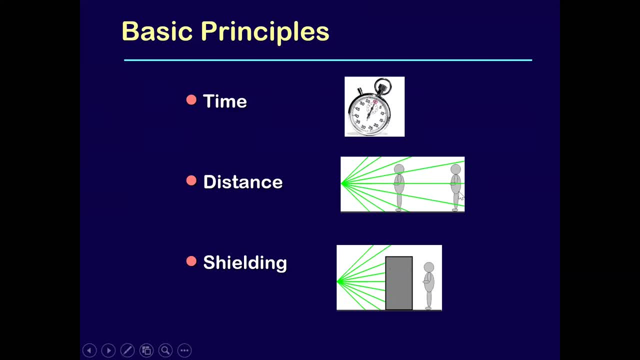 at one metre. a person goes and stands at two metre, the intensity reduces by one fourth. 25% reduction, sorry, 75% reduction. He gets only 25% dose. It's very advisable. So when we are doing an interventional procedures. 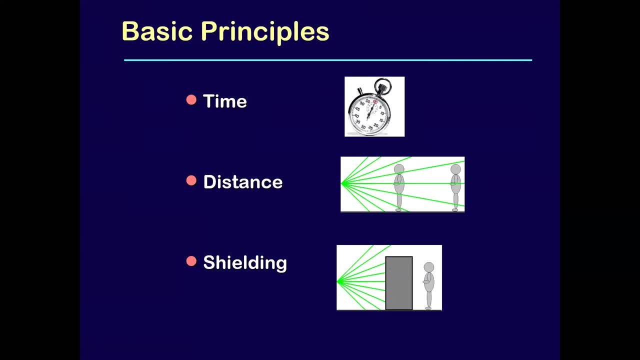 Okay, Of course you cannot stay at two metre, but try to stay at least 45 centimetres or 50 centimetres. use your hands to do the procedure and nowadays you have robotic machines to do robotic surgeries. So similarly, in the C arm and other things, there are a lot of radiation protection gears. 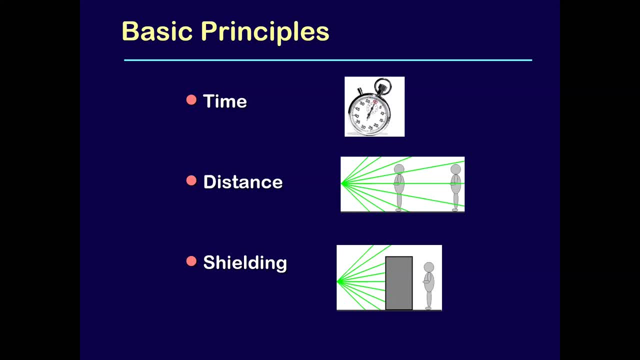 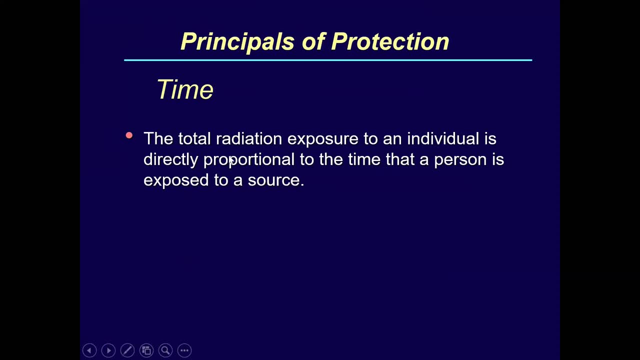 You can wear those radiation protection gears when we have to be very close with the patients, or you can make as much as distance possible, Okay, So the total distance, Okay, Okay, So the total radiation exposure to an individual is directly proportional to the time that 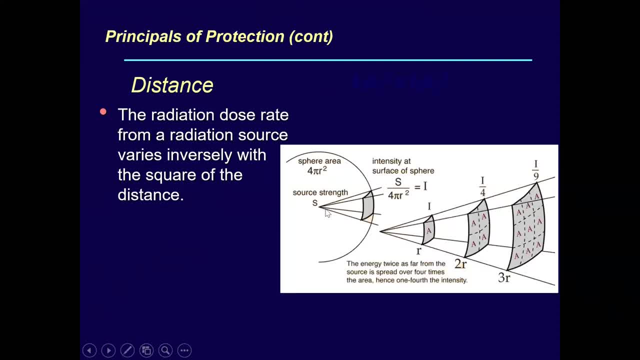 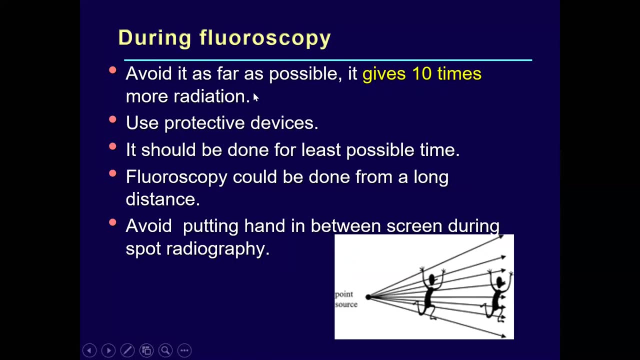 a person is exposed to the dose And similarly, as I told, if you increase the distance by one metre extra, you reduce the intensity by 75% reduction. So again, when we use fluoroscopy, again a fluoroscopy is a purpose where avoid it. 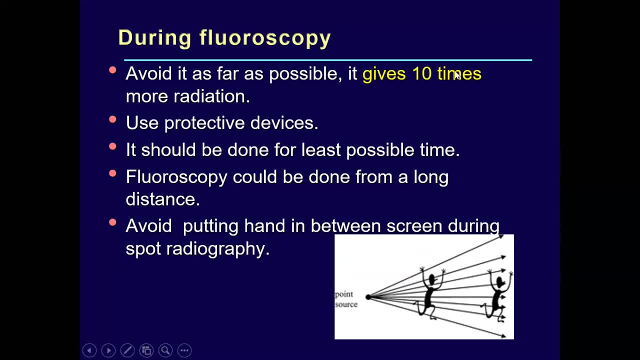 as far as possible, because a fluoroscopy gives you 10 times radiation that you can't get from radiation, And so if you want to do that, then you have to use the fluoroscopy. The fluoroscopy is a more effective way to reduce radiation than an x-ray. 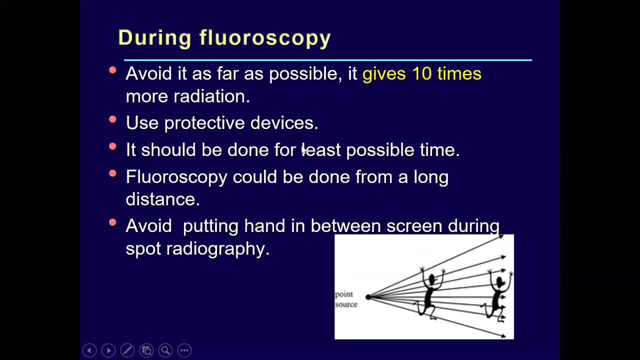 And whenever you are doing a fluoroscopy procedure, please remember to use protective devices like the lead apron and glasses if it is required. And so when you look into the X-ray tube shielding, you see this is the X-ray tube. 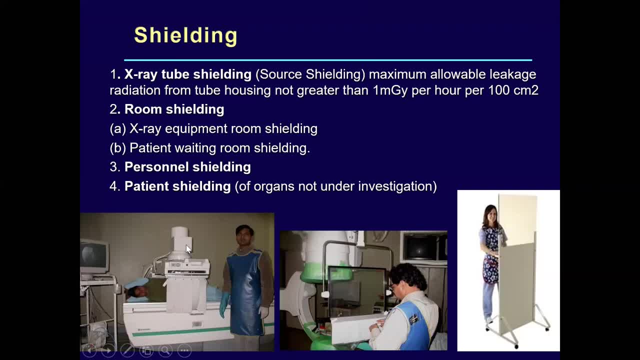 This X-ray tube when they do for servicing and other thing, they have to be housed properly on the shielding environment. There should be no leakages And if a patient is getting exposed to radiation they have to be housed properly on the shielding. 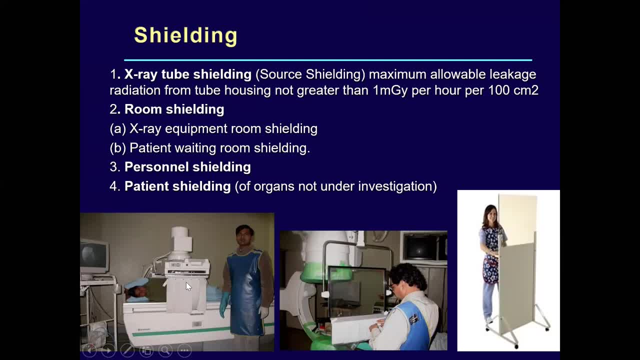 environment. There should be no leakages. you see, these papils, they all have radiation attenuations. So or you can have a bedside trolley with a lead glass. This, you see, it is a little little opaque, is less, but you can still. 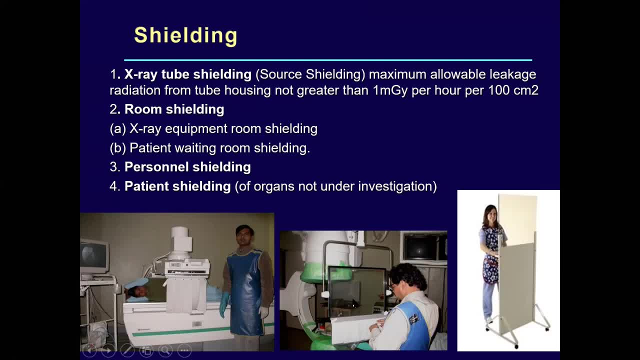 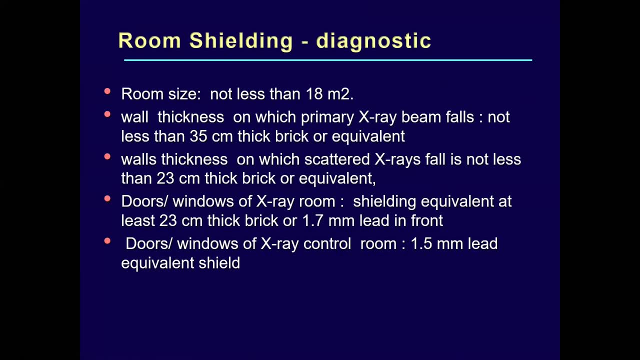 visualize them. This is not an ordinary glass. This is a lead glass. It has a high atomic number property to attenuate the x-rays. So there are definite guidelines set for radiodiagnostic and radiotherapy purposes. The guidelines set for a radiodiagnostic purposes is that the room size 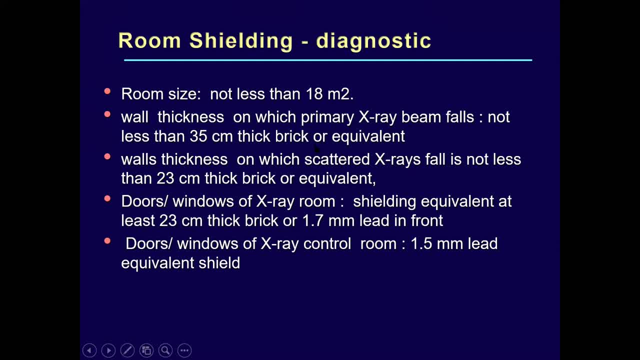 should be minimum of 18 meters square And the wall thickness should be of 35 centimeters. brick brick wall 35 centimeters thickness And the door: there should be no windows. If there are windows and doors, they have to have a wood with two millimeter lead coating. So many of the x-ray. 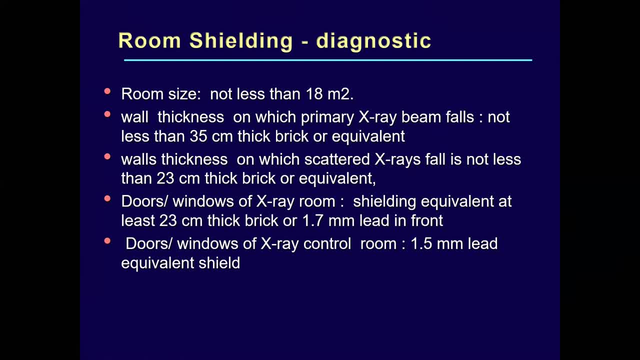 exposures. when you see beyond the doors, they will have two millimeters of lead sheet embedded in between the doors. And also it is important, not only the doors have two millimeter of shield, the frame, the frame where the door is going to close, the frame also will have two millimeter lead all. 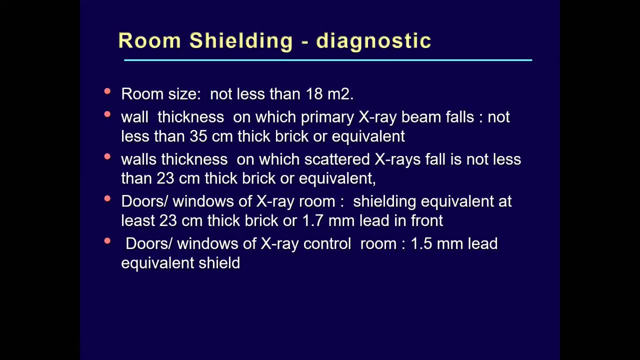 around. That is how the radiation will be reduced for the persons or for the public who are walking across the radiation environment, Whether it may be a OT C arm in a OT or a x-ray machine installed in the radiodiagnosis department. 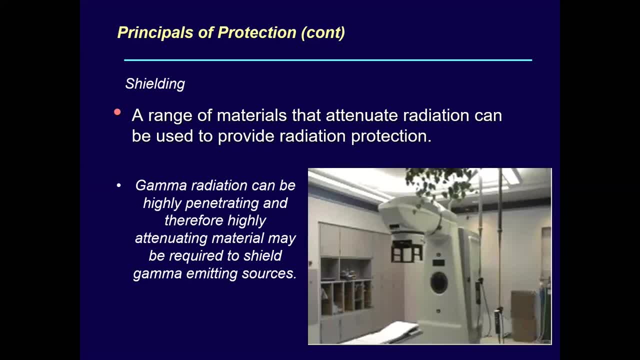 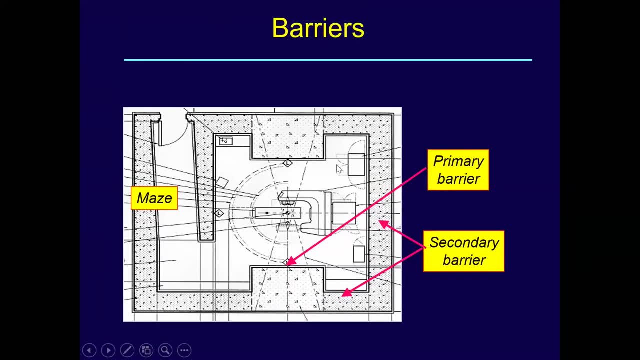 But when it comes to therapy purposes, the radioactive for a telecobalt machine is very large. Look at this. This is a room layout. The machine is housed here and the control console is here. This is a maze wall. A person in radiotherapy doesn't enter. 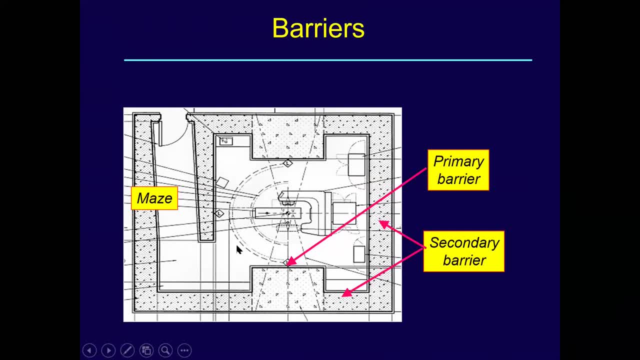 the machine straight away. He undergoes through a maze wall in order to enter the room because the radiations are very highly powerful and it have a very large intensity and you need concrete thickness of sometimes a high energy linear accelerator. You need concrete thickness of one. 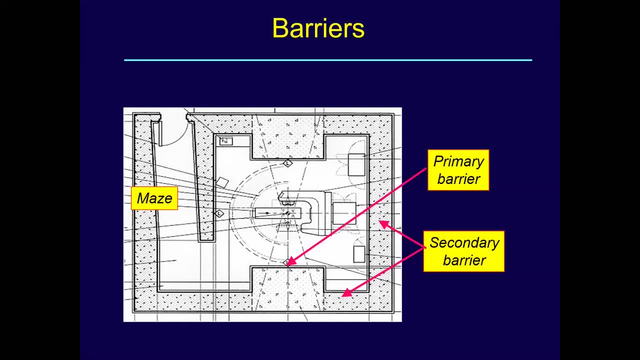 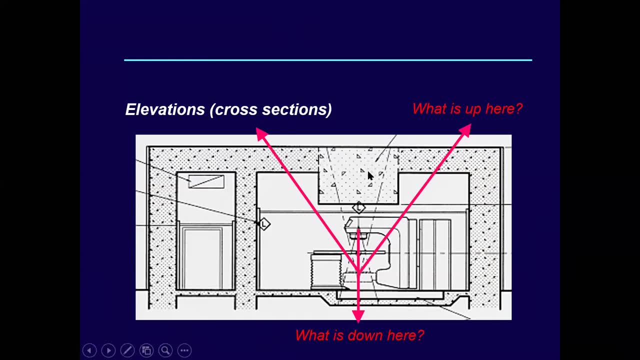 meter. Remember that One meter of concrete Building such a kind of a huge facility is very, very protection. and even a bomb falling, nothing will happen in this room. So it's in a much boot room, but I got that for radiotherapy exposures in order to have a safe. 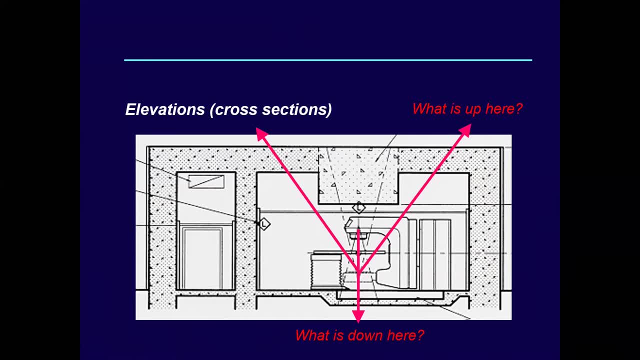 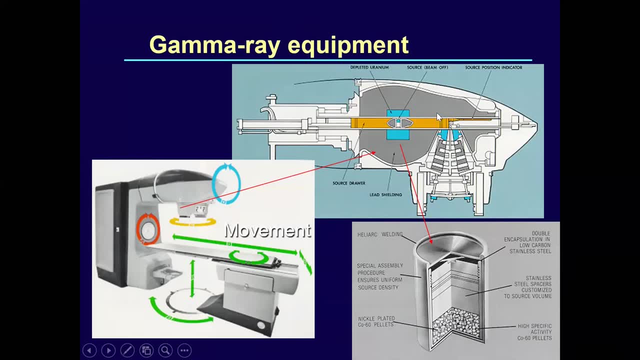 radiation delivery to the patient and the radiation workers who are administrating that radiation doses, because the radioactive material is kept in there in this big housing And this source moves from this on to switch off to on position to give a radiation. I'm not going to go deep into this. I 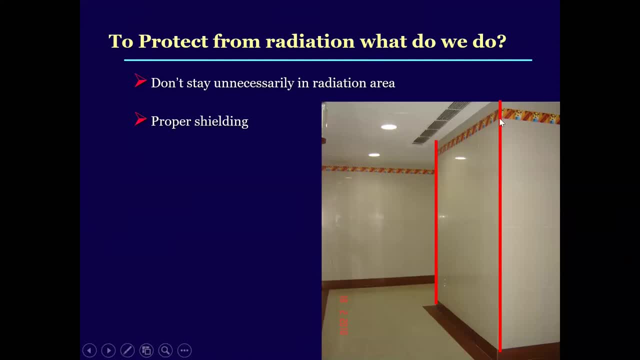 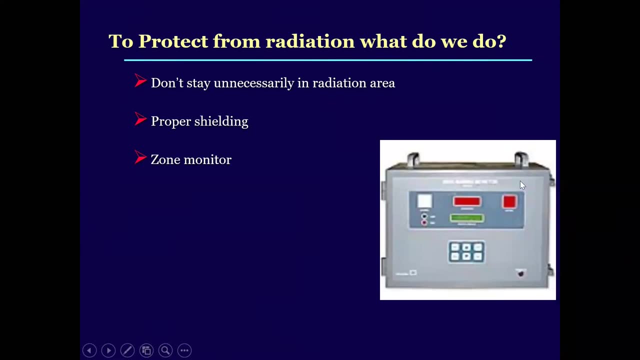 just tell you: show the rooms. The walls are and there will be always indicators like gamma zone monitors are installed in most of the radiation environments which will be give beeping and red alarms to show whenever there is a radiation And if you see any. 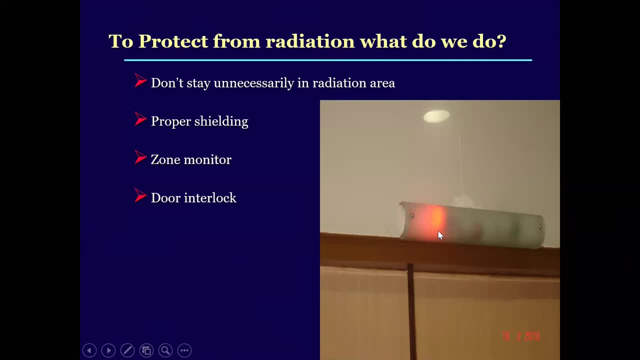 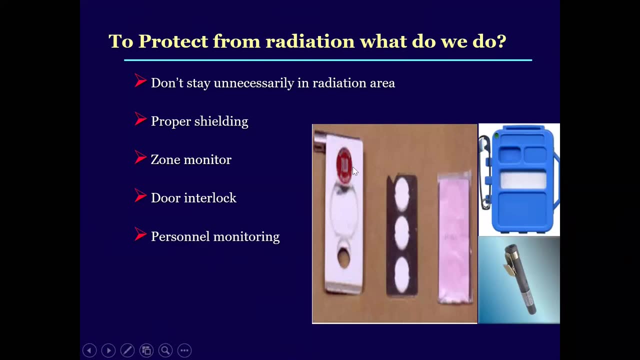 radiation environment. that will be red, green and yellow color indicators And there are variation, various radiation personal monitoring devices. One of them is thermal luminescence dosimeter, or we call it tld. before TLD, We add film badges. And there is one more thing: Parkvision. it all, This pocket. 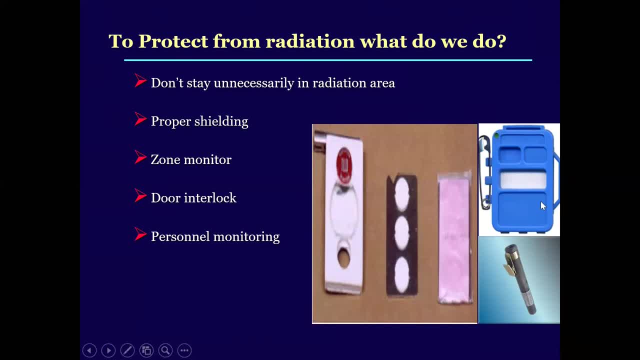 TLD is used when you think you're going to do a radiation intervention where you may get that more radiation. Otherwise, for general monitoring, we use that TLD badges- Thermal luminescence radiation monitoring badges. There are three TLD shelves here And there are different waters. This is a light copper filter. This is a plastic filter. This is a communautar. 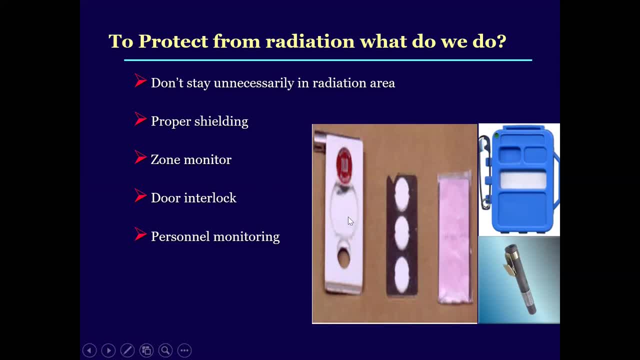 filter. So the radiation attenuates by these filters and the intensities are read in such a way to know what are the radiations produced by X-rays and gamma rays and beta rays. And this is the radiation symbol Generally. I will again elaborate the symbol dimensions. 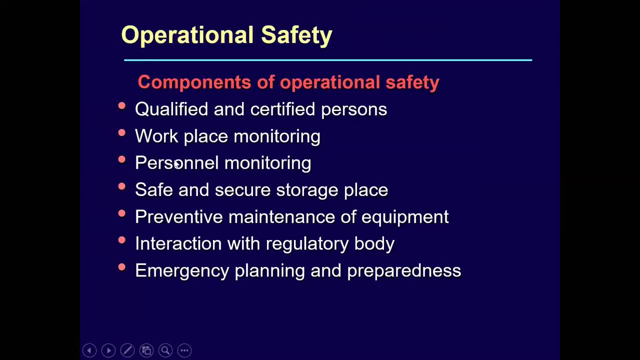 and other thing later. So radiation has to be operational by only qualified and certified persons. Work space need to be monitored, which we call it as a radiation survey of the environment. Personal radiation monitoring is done by wearing film badges, and these badges have to be kept. 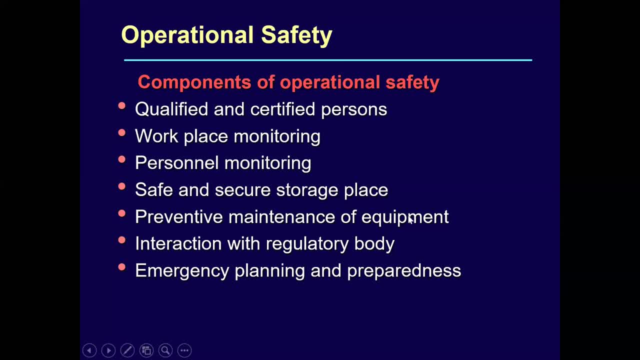 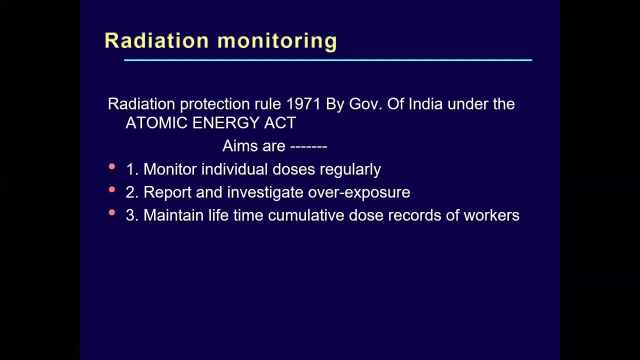 on a safe place, non-radiation zones. Preventive radiation QAs are important. International guidelines have to be followed, regulatory guidelines and there should be always an emergency plan for the preparedness in cases of radiation damage, radiation accident, So So. 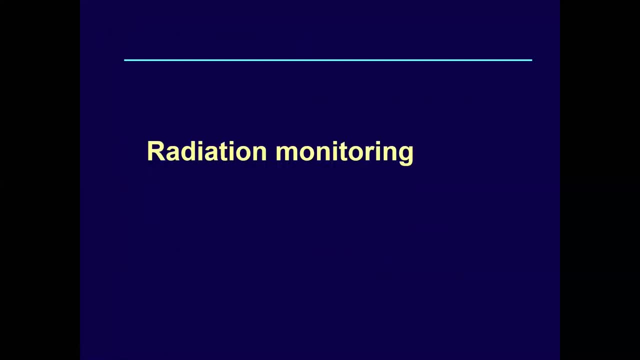 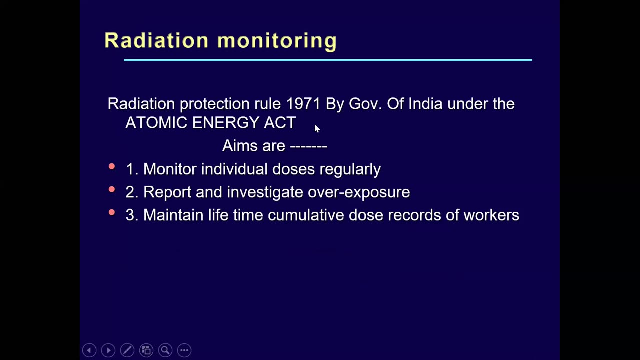 again. I would like to take another five minutes to talk about radiation monitoring, because there is an act by Atomic Energy Regulatory Board 1971 that we are mandated to do Again. I want to tell all the residents one more thing, In case you are working on a sea arm. 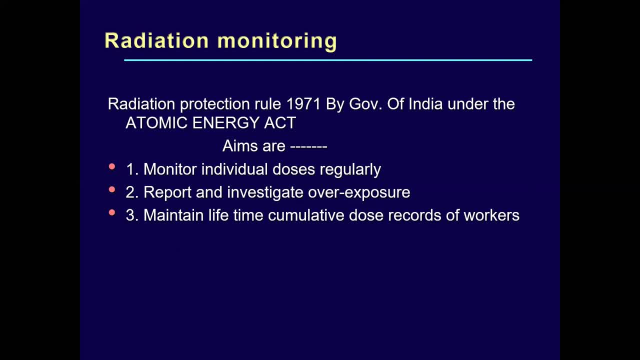 or a radiation environment posted more than one month continuously. you should get a film badge issued and recorded. Remember, these film badges are one time issued in your life time and your personal monitoring number is carried over wherever you go in the globe to have your radiation dose accumulated. to know your radiation accumulated during your 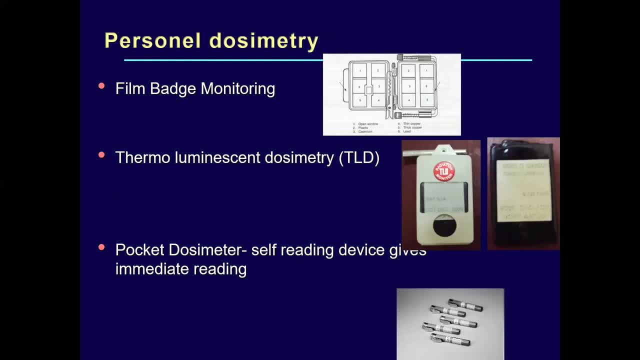 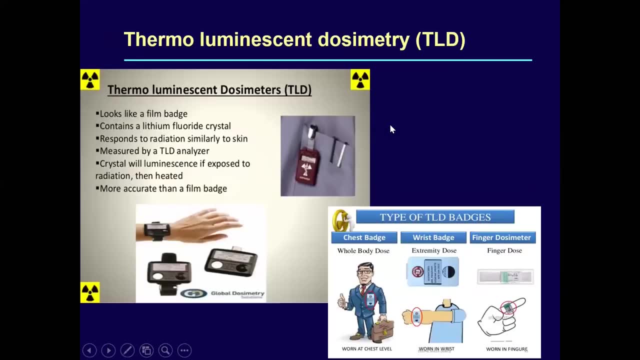 lifetime. So, as I told you, these are the radiation instruments: thermoluminescence pocket dosimeter and film badge, and there are different wrist badges, as well as forehead and finger badges. People who work very closely with the radiation instruments need to have a film badge issued. 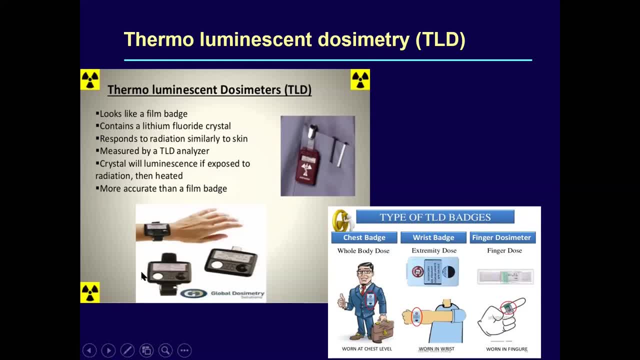 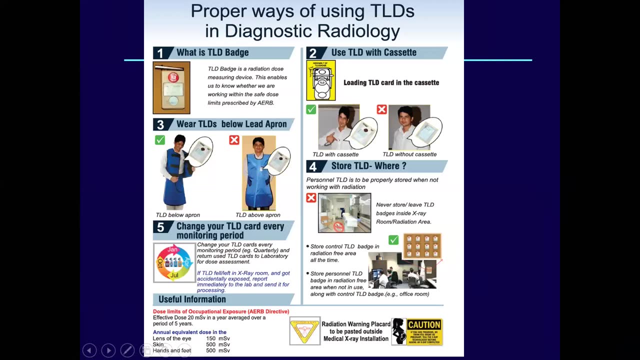 People who work very closely with the radioisotopes, like nuclear medicine, that they used to practice with apart, along with the chest badge, they, in addition to that, they have a wrist and a finger badges, if it is appropriate, And these badges have to be bad about the apron. 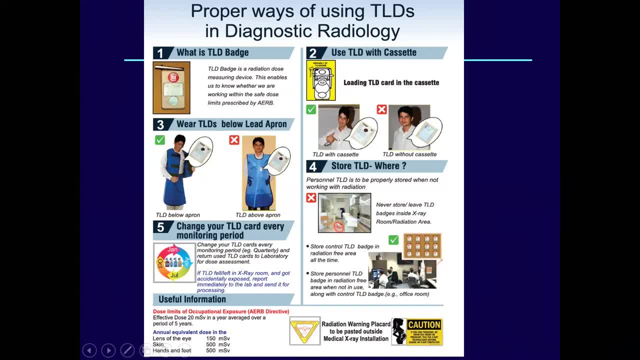 not inside the apron. Okay, And radiation symbols are always. these are radiation symbol from my x ray mission and this is: should be placed In all x ray units, whether it is a C arm x ray or CT scanner, and pregnant females should be warned not to sit close to that and in case they are going for a x ray examination. 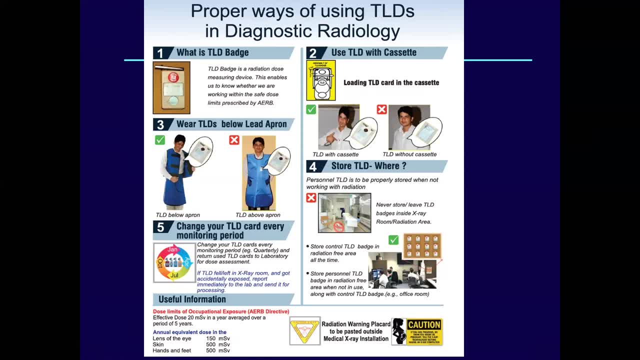 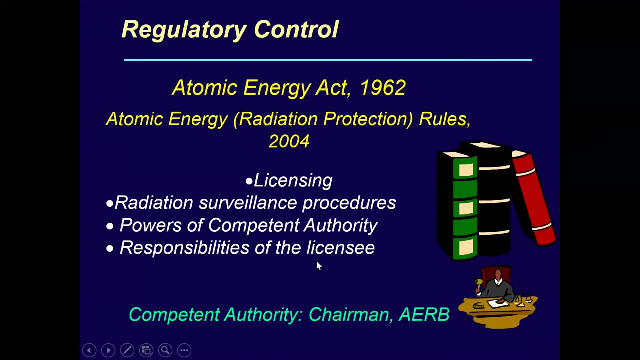 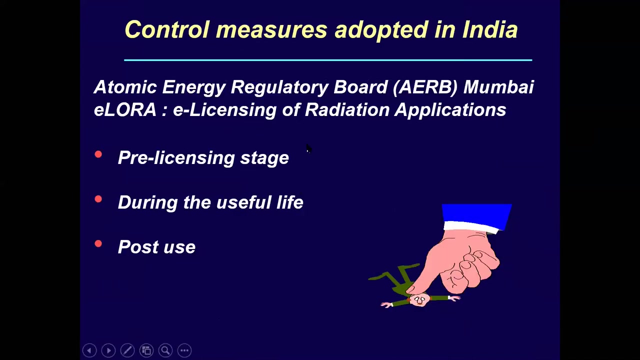 they have to declare and requisite counselling need to be done for any suspicious or confirmed pregnant females before radiation examination. So by the act of atomic energy regulatory board, And if we don't stipulate into the guidelines and don't obtain responsibility of licences and safe practices, they can punish us and they can cancel the license and the institute. 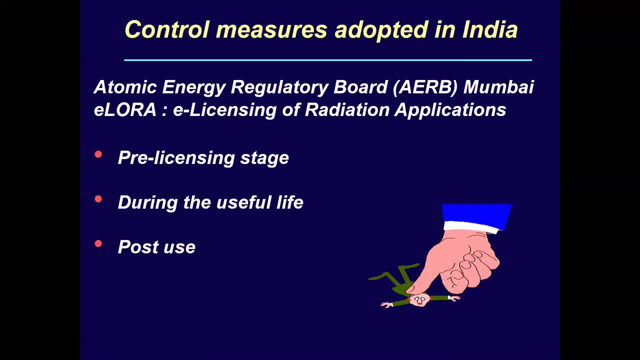 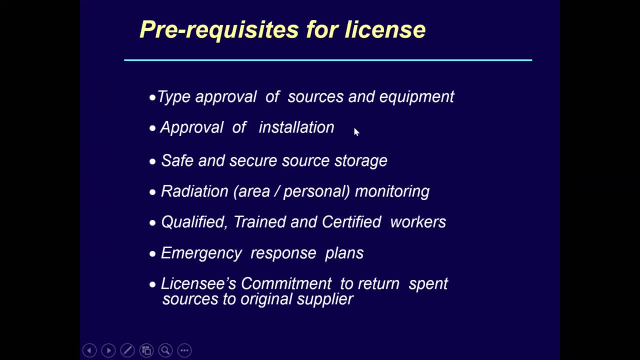 can be debarred by using x rays for diagnostic practices. So for that we need to have qualified radiation safety officers in the Institute and that has to be a radiation safety cell. they have to keep monitoring the radiation the environment in the hospital by surveys. personal monitoring always undermine device, which is bad curve. 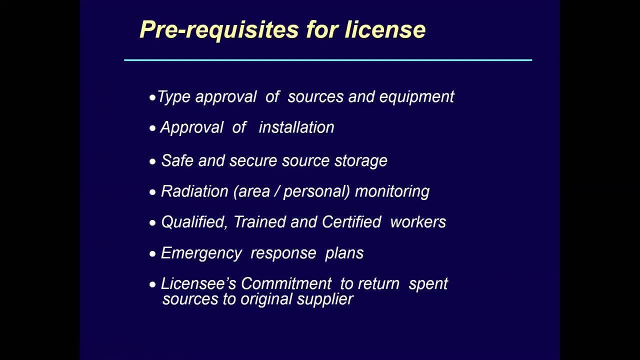 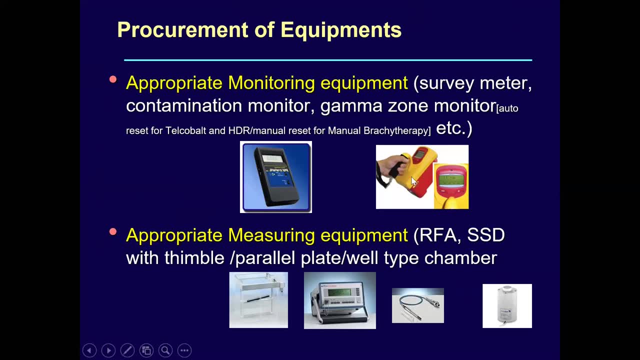 of reaching levels decrease, which is grainy, is normally aggressive or also worse during those related epidemiological events. Nevertheless, there is a failure to to rarely showing out monitoring and quality assurance programs. So there are various instruments for personal monitoring, various instruments for survey. 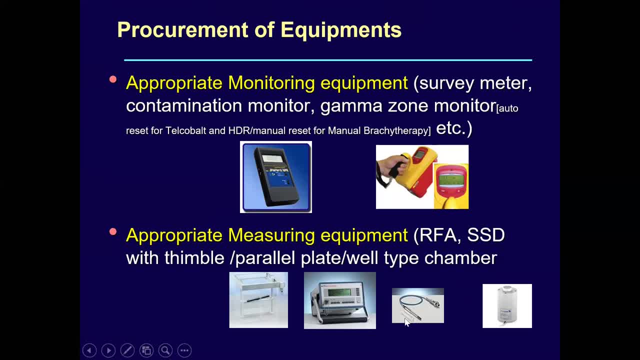 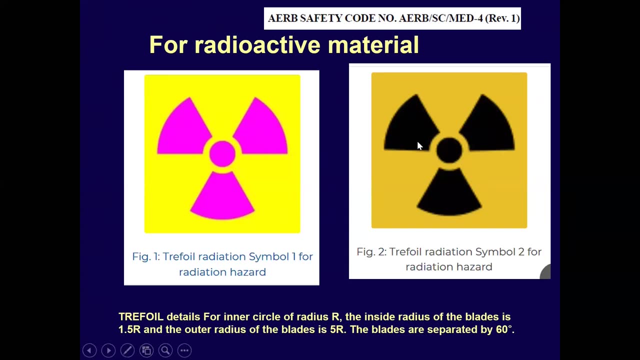 which is GM gamma survey meter, and ionization chambers for measuring absolute doses from a CT or from a therapeutic machines, or for a blood irradiator, for that matter. So these are the two radiation symbols. Radiation symbols can be in pink color or black, and they have to be segregated by three. 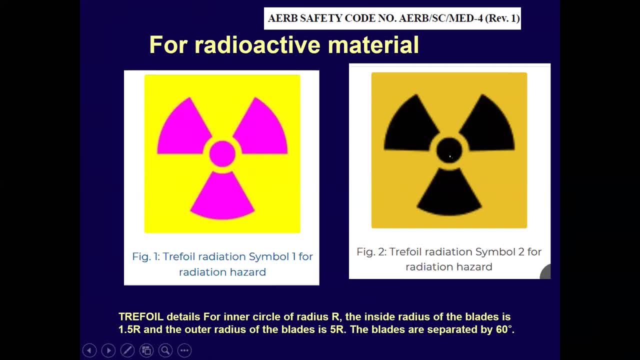 triangles like this and the radius, the central radius, is 1R, means from this to this is 5R, So this is four times the radius of this. So the proportionality of radiation is to be adhered. and each of these blades, these, 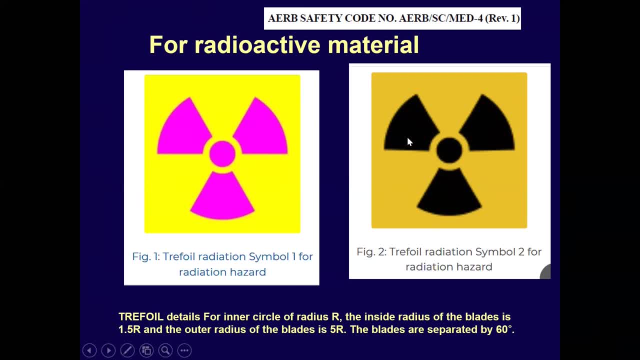 fan blades have to be separated apart by 60 degrees. So three blades and three empty blades. These empty spaces together covers 360 degree. So these you cannot just draw by a manual sketch without adhering the principle when you put a radiation symbol.